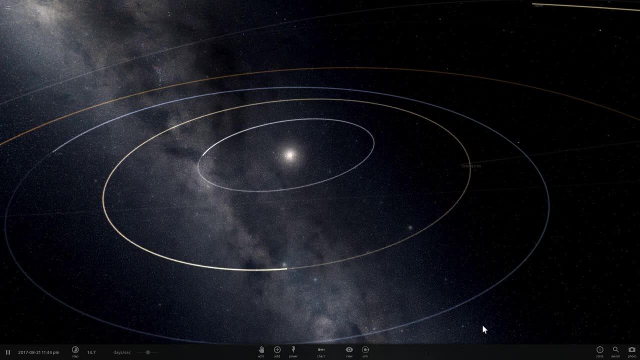 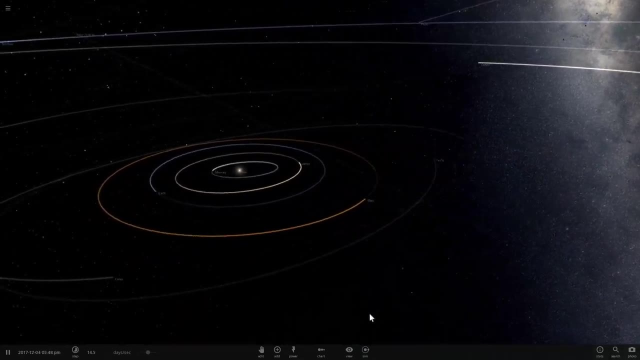 And welcome back. This is Universe Sandbox 2 or Universe Sandbox Squared, and we're going to be using this game to try to well, first of all, explain what quasars and blazers are, but also just talk about their structure, their features and so on and so. 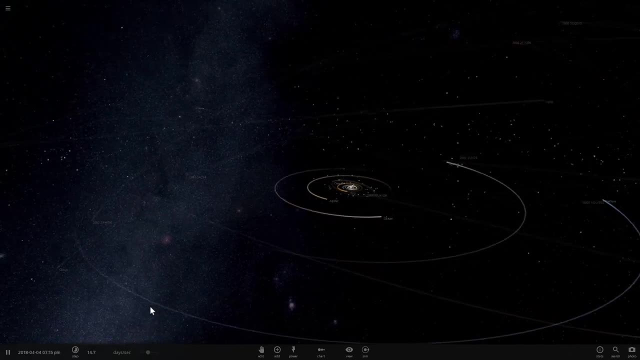 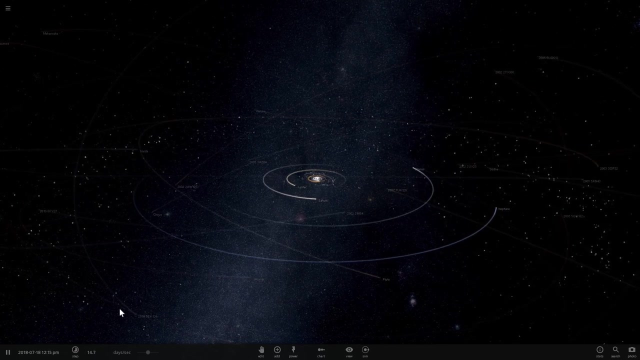 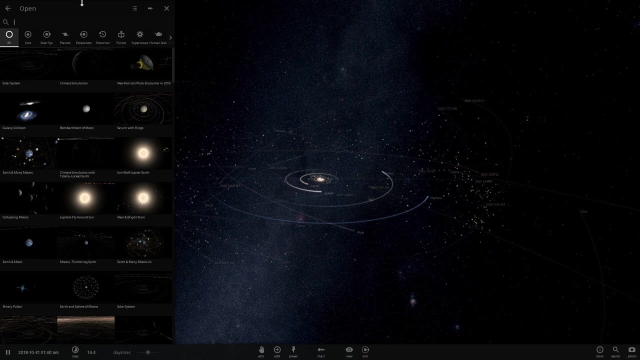 forth. Unfortunately, neither Space Engine nor Universe Sandbox 2 actually have any quasars or blazers or any other AGNs or so-called active galactic nuclei objects in their repository. So here, even if I go through all of these, I will not find any quasars or blazers or anything like. 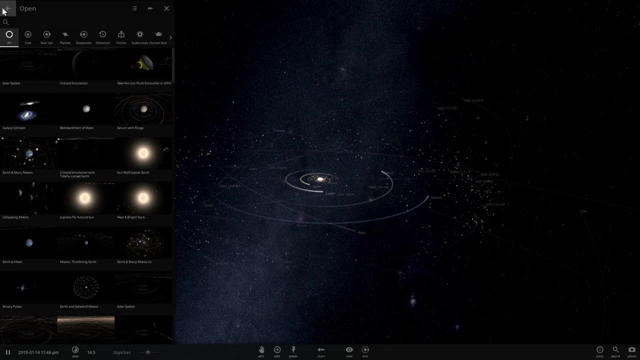 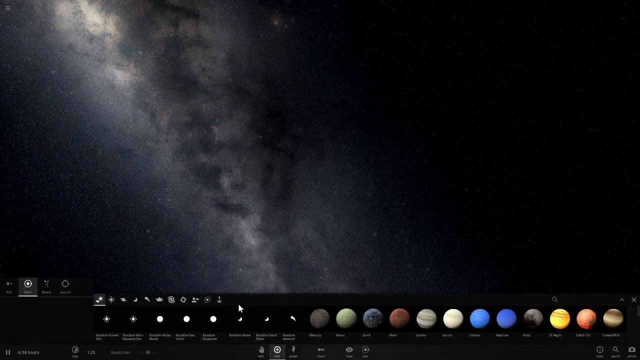 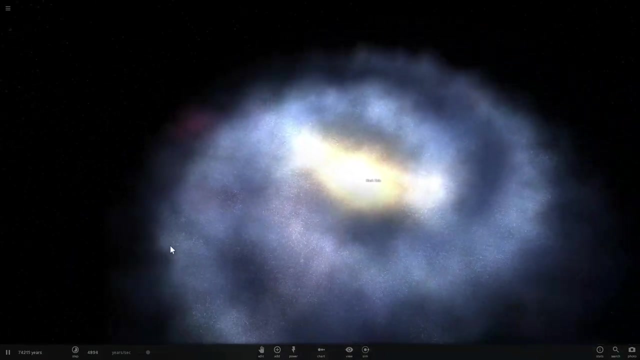 that. So I have to make one from scratch, And this is actually good for us, because that way you'll get to visually see what they are and how they basically are made. And I guess we should just start with the basic definition. So quasars and blazers and radio galaxies are all galaxies. 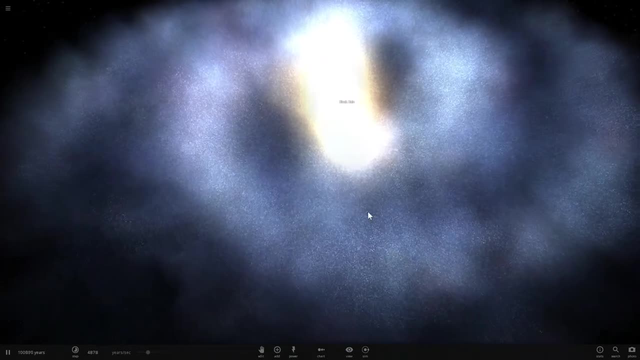 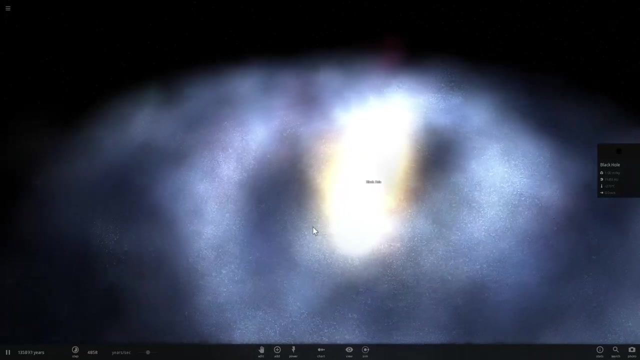 They're not just stars. They're actually very, very large galaxies that have a massive, a super massive black hole right in the middle, right at their center. And this is what makes them different, actually, is that they're um, they're called active galactic nuclei because, if you were to go, 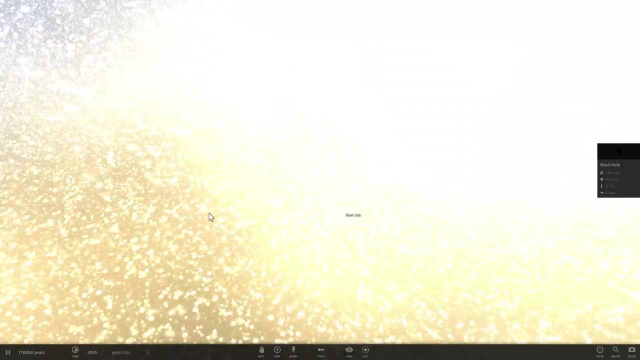 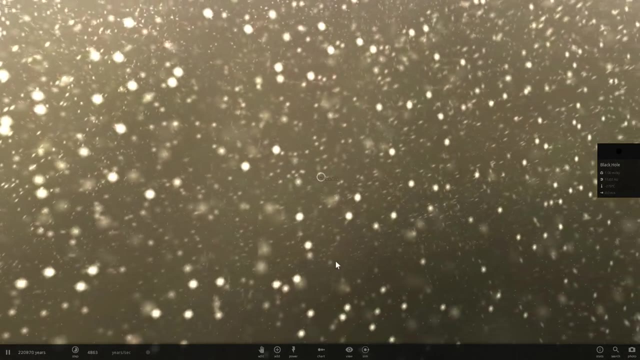 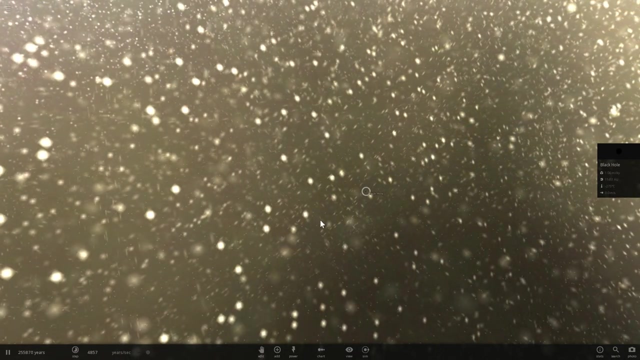 really, really close to this black hole. what you would see is that this black hole is actually absorbing and eating up and basically destroying a lot of various uh stars, a lot of various uh matter, And it's just kind of taking it all in and uh it a lot of it starts accreting around. 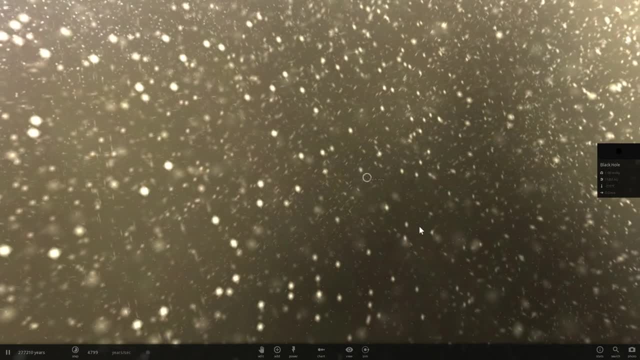 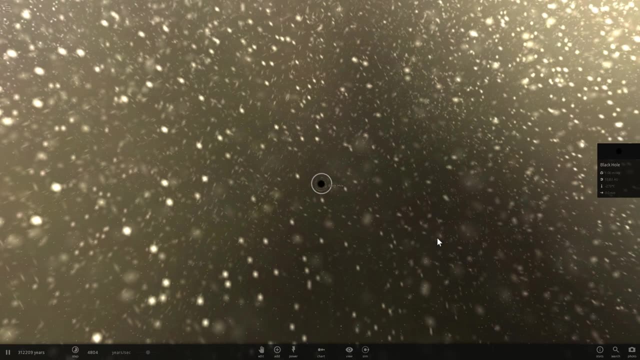 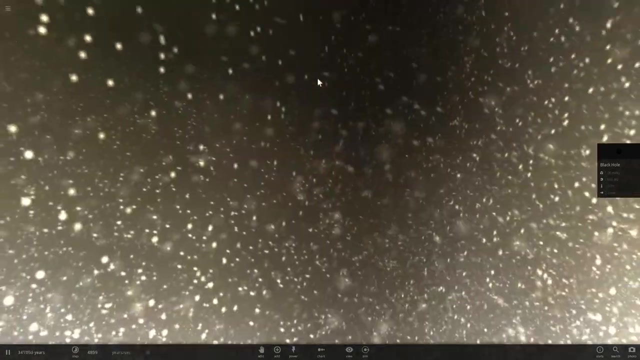 it and creates an accretion disk. And because of this accretion disk, uh, so much energy is produced that uh, and also so much uh electromagnetism is produced that a lot of the magnetic powers, magnetic forces, create these two sort of rays, going sort of up and then down, and these rays 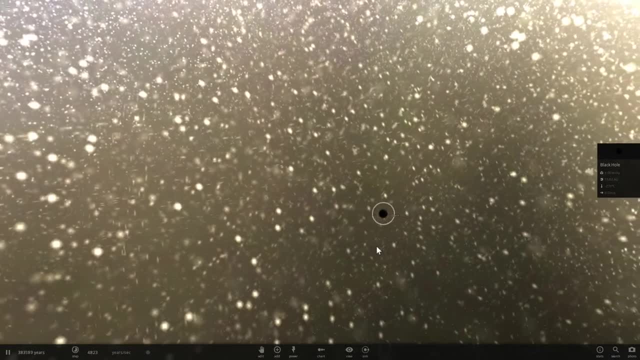 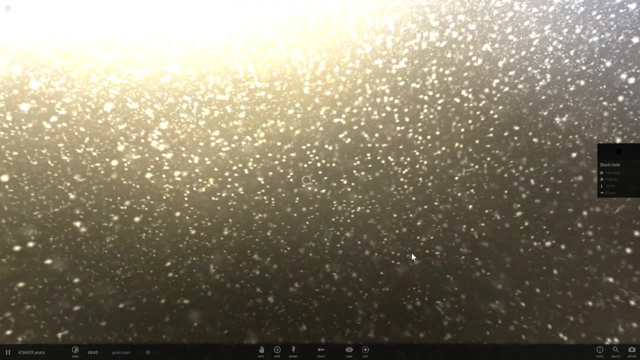 are what are what we're actually interested in. but to make those rays happen in this game, we're going to have to cheat a little bit and use pulsars. I'm going to show you how we're going to do this in a second. well, let me just actually show you what I mean by this. so imagine so this. 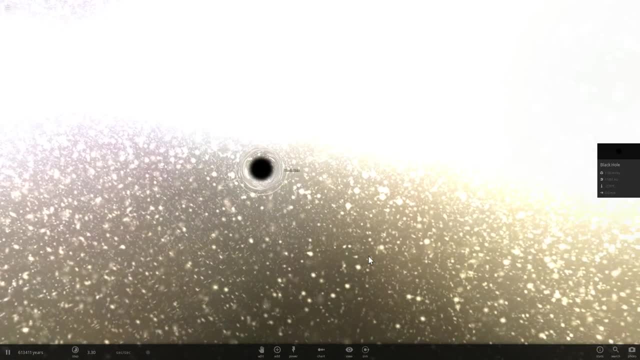 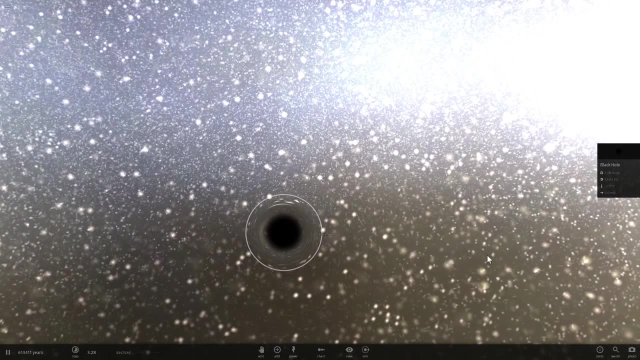 is a black hole right here now. earlier on in the creation of every galaxy, every galaxy goes through the stage when there's quite a lot of matter in the middle. a lot of the stars come really close to the central black hole and as this black hole grows in size, a lot of this matter gets absorbed. 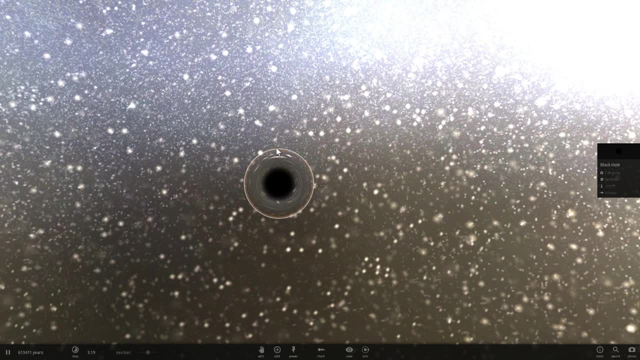 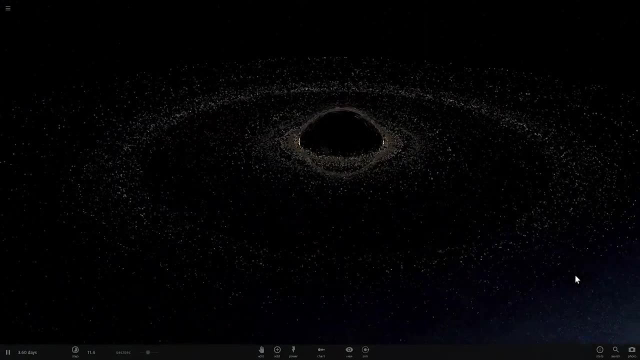 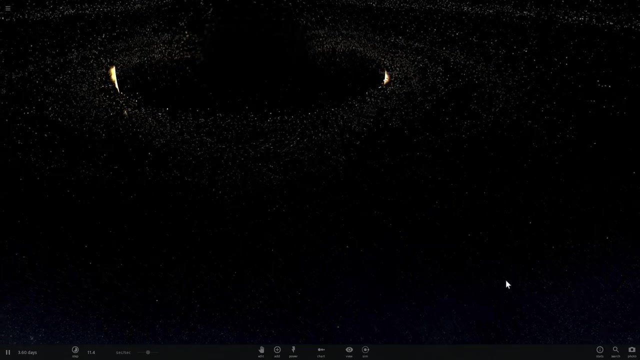 it basically gets sucked into the black hole and some of the leftovers start orbiting around, creating an accretion disk. an accretion disk that sort of possibly looks something like this, except it's much more massive, much more energetic and much more- uh, better looking as well something. 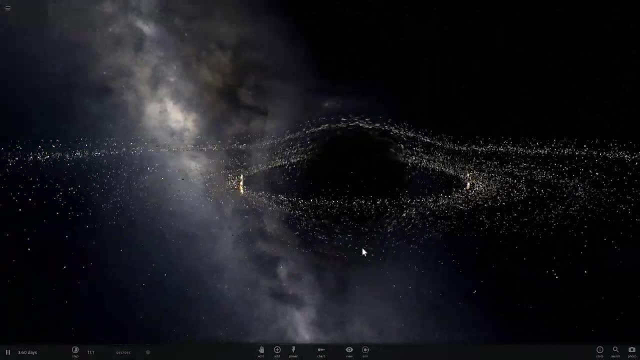 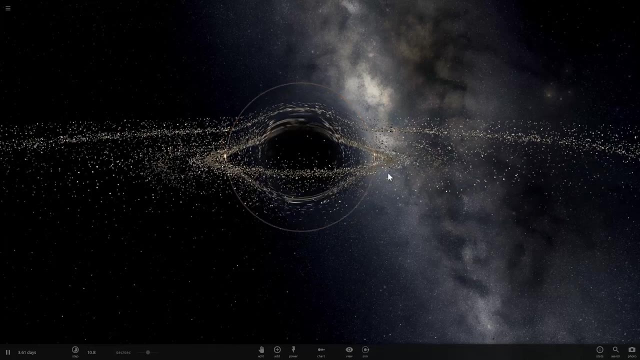 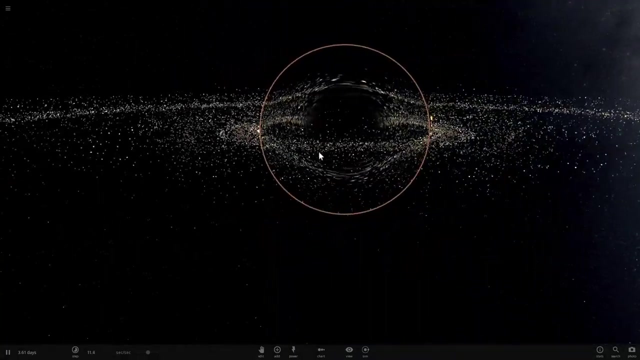 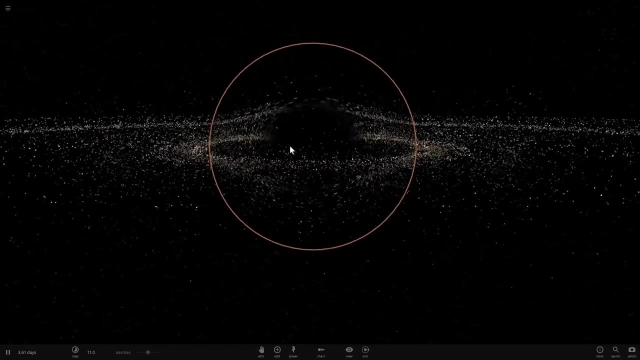 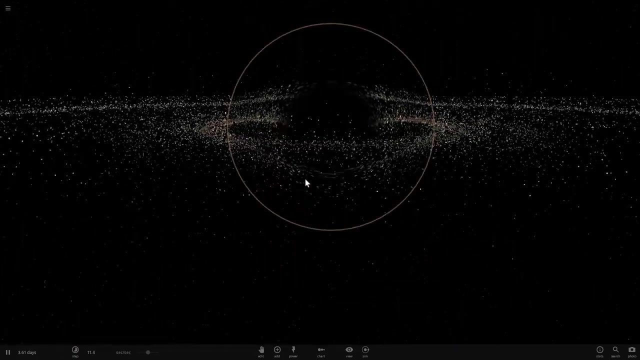 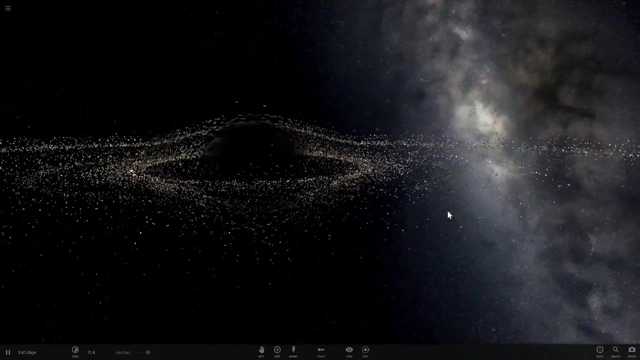 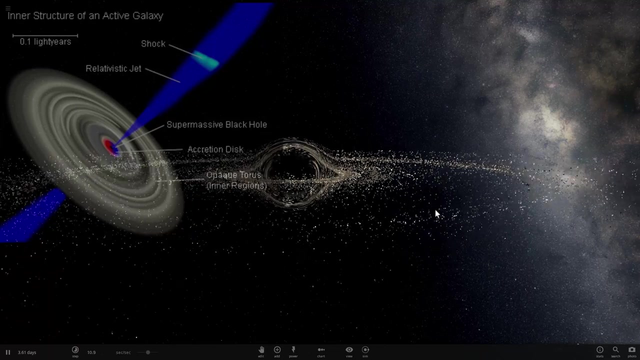 that we may have seen in the movie called interstellar, now foreign. unfortunately, we're still not 100 sure why this happens and how it exactly works, but we know that it happens because we can observe it, uh, in space and anyway. so this is the black hole that we have. 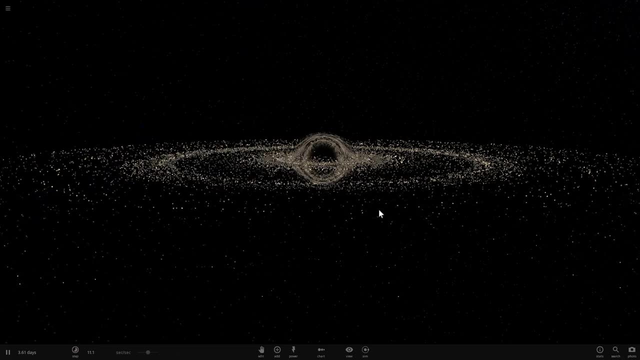 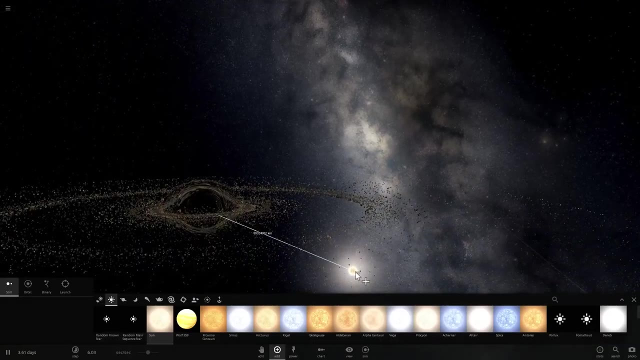 with the accretion disc, and what happens next is really interesting. so let's just actually throw a few stars into this just to give you an idea what's happening. so what I'm going to do now is I'm just going to place a bunch of stars around this black hole- uh, simulating, uh an. 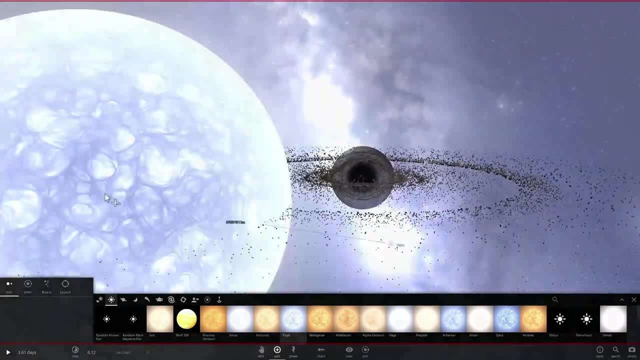 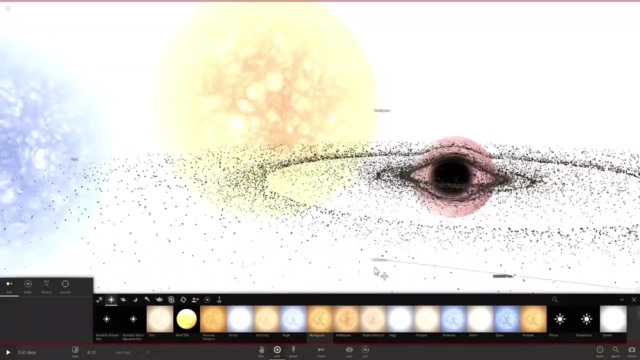 environment where many of these stars didn't really get really lucky. or even this big one, uh didn't get very lucky and got basically, uh, sucked into this black hole. so there's some of these stars will be very, very large and this will be quite interesting to observe. so basically this: 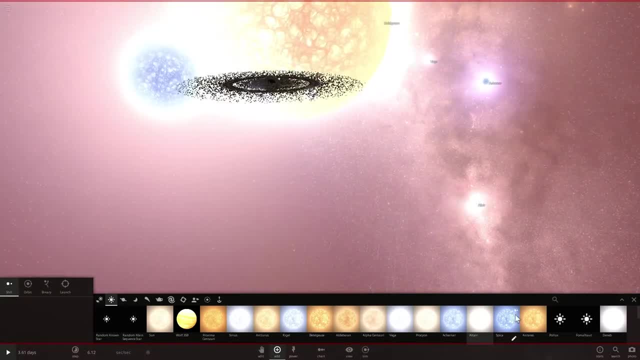 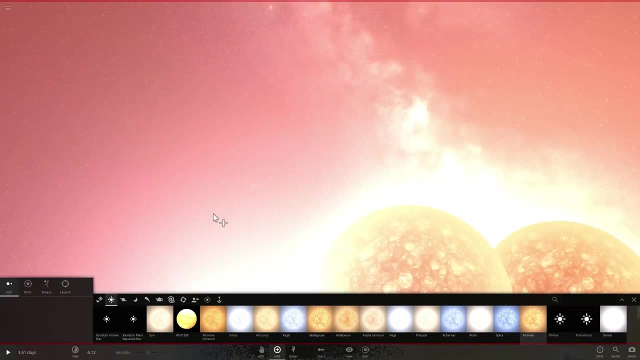 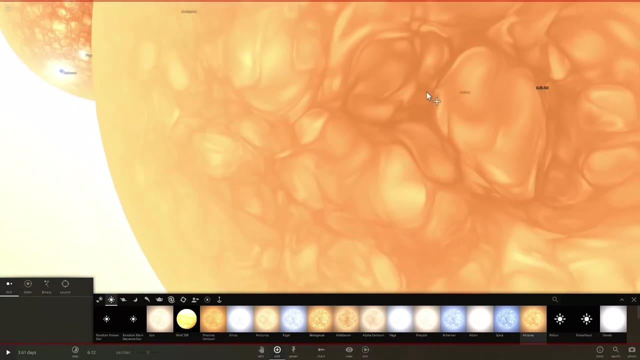 is a simulation of what an active galactic nuclear looks like, and this was very common earlier in the universe when a lot of the early galaxies were basically uh saturated. and they not only saturated, they basically had a lot and a lot, a lot of these um early stars that basically didn't get lucky like 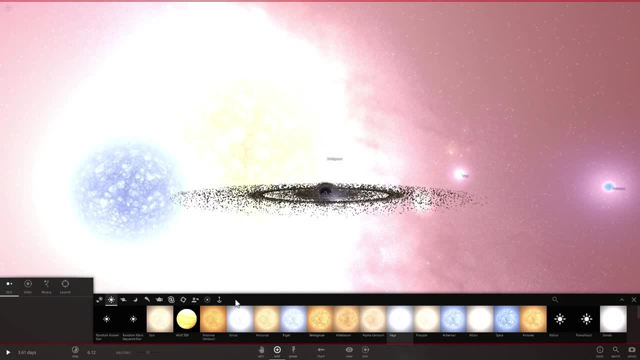 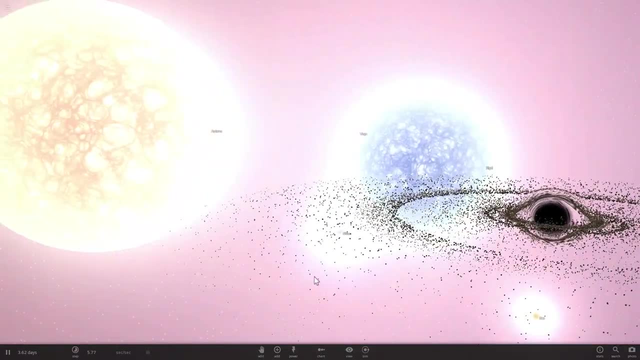 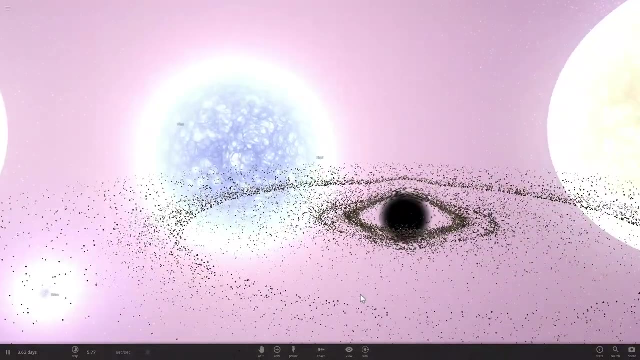 I said, and ended up inside the black hole. so we're going to continue the game, we're gonna unpause it and let's see what happens. so as these stars approach the black hole, they will most likely- or not most likely, but very likely- get sucked in and get destroyed as well, and as they get, 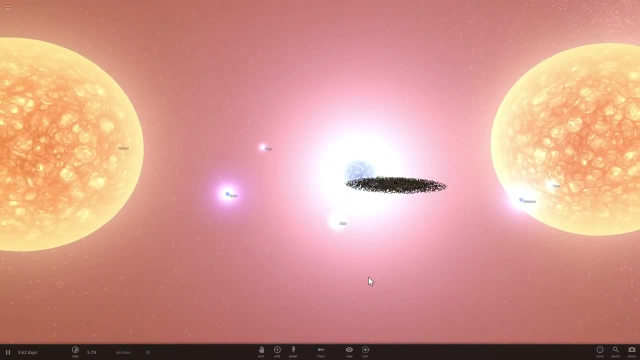 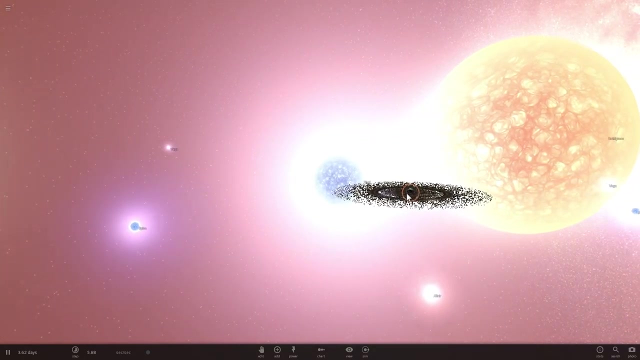 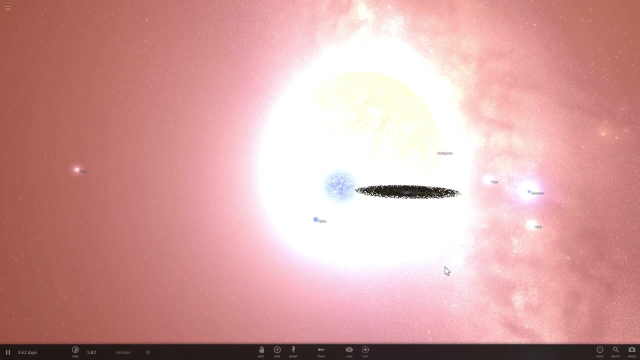 destroyed, they release such a massive amount of energy, um that, uh, these- unfortunately we can't really simulate this here, but we're going to do this in some other way- that, um, these two streams, going up and going down, increase dramatically, and this is why quasars, Blazers and all other active galactic nuclear objects have such a a variable. 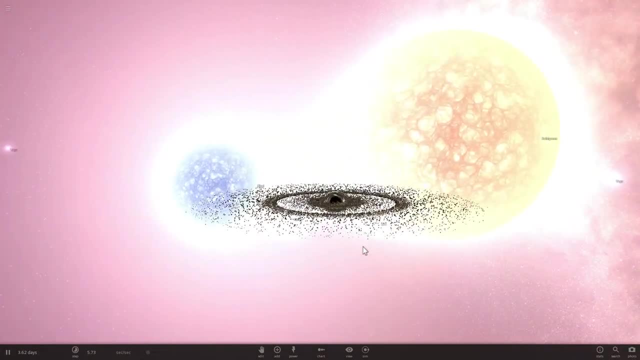 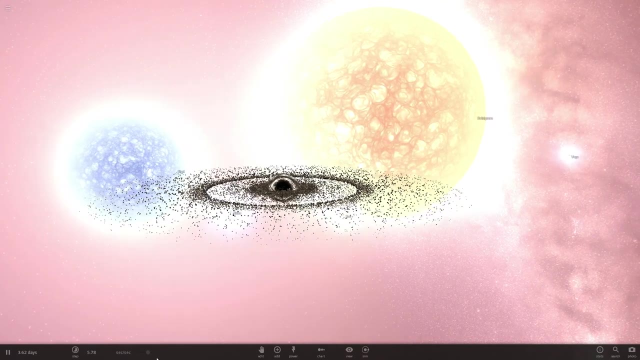 luminosity. in other words, they actually change the luminosity depending on how many stars are being absorbed by this particular black hole and, in reality, all of these active galactic nuclear objects work exactly the same way. there's a central black hole that is very, very massive and it suddenly 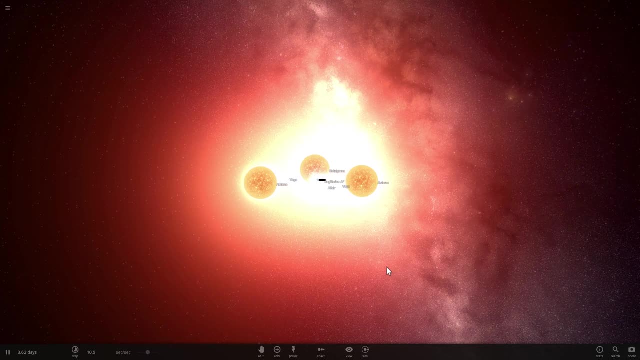 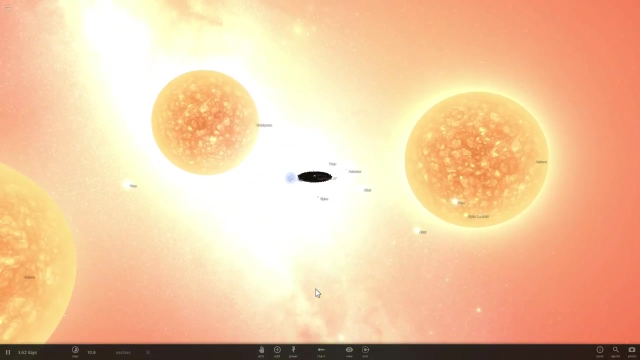 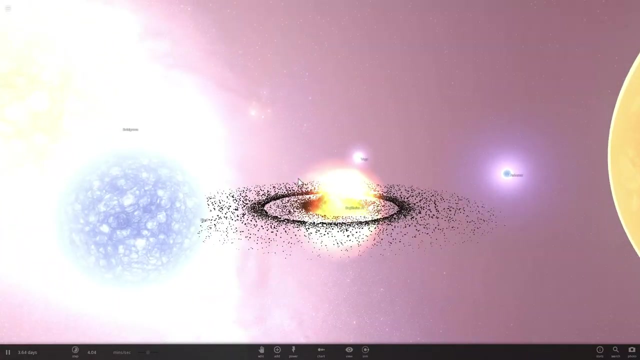 gets quite a lot of material get that gets sucked into it and basically gets destroyed in the center, and the energy that's created by all of this is then projected um in two directions from the Galaxy. so here comes the first explosion, and unfortunately it doesn't really do the whole. 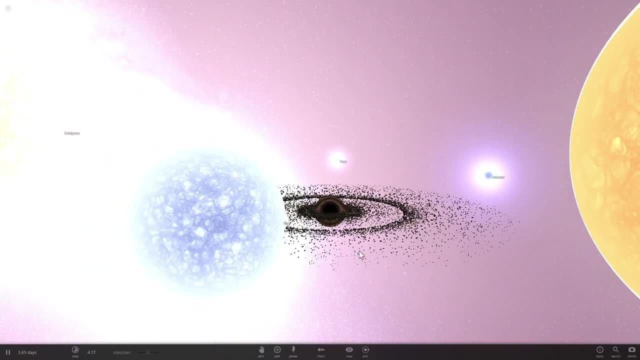 jet thing that you would see in real life. it just kind of explodes as soon as it approaches the black hole, and the very big black hole they just break up into smaller. I really want to wish I could just find it there that I could at least buy the Giants. at least buy them at least. 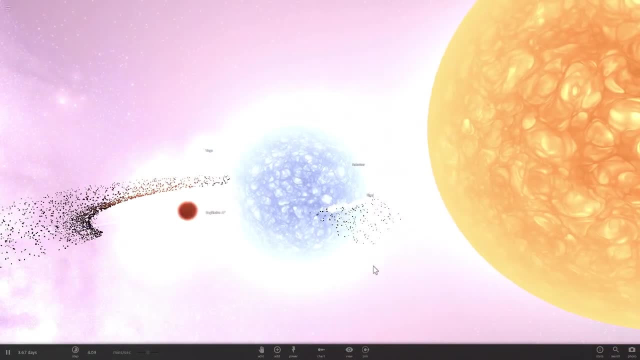 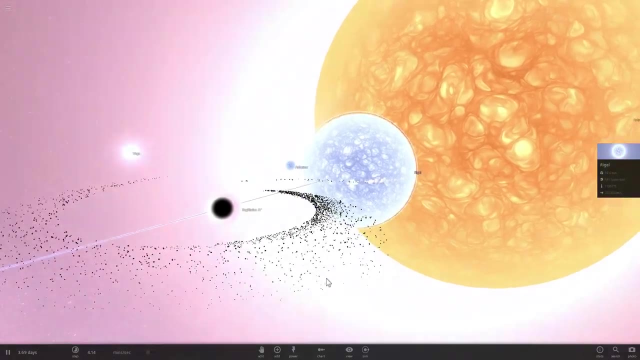 they start approaching the black hole and no, where are you going? come back. oh, it flew to way past the black hole. it's probably going to collapse with Antares and there might be actually a supernova afterwards. but, as you can see, they've absorbed quite a lot of the uh particles that I 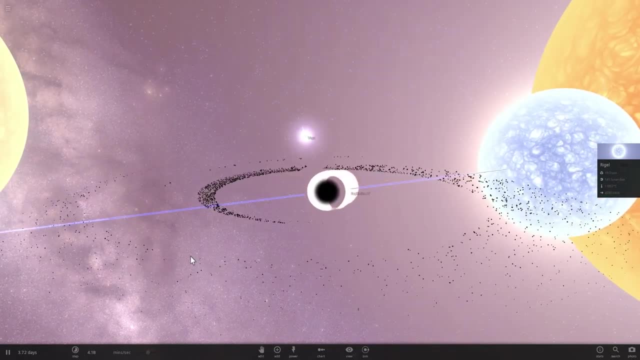 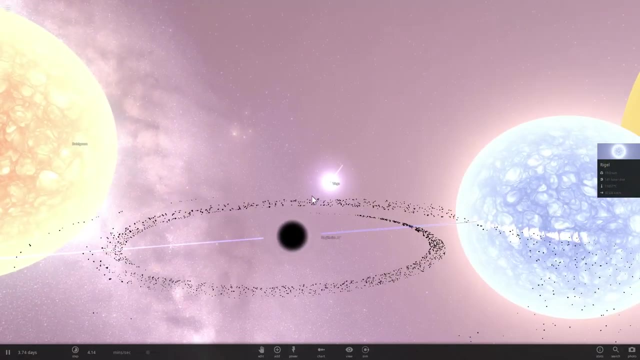 had around. they were representing the accretion disk which actually accelerated my game. so here comes the second explosion and look at that, the radio is coming back. it's coming back for another spin because the gravity of this black hole, which is actually exactly the same black hole as in the 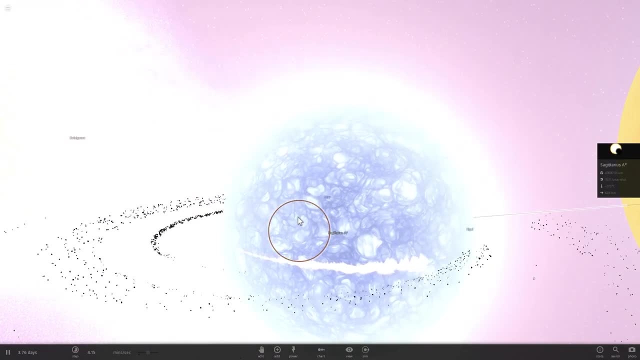 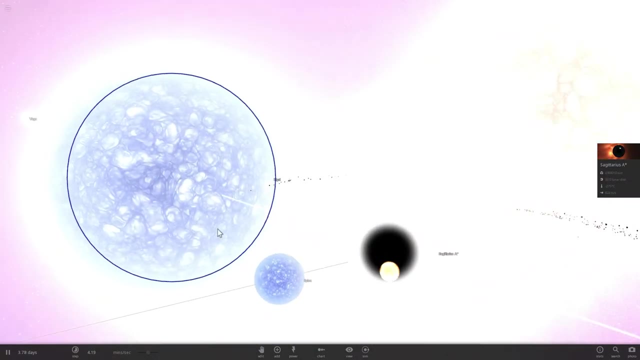 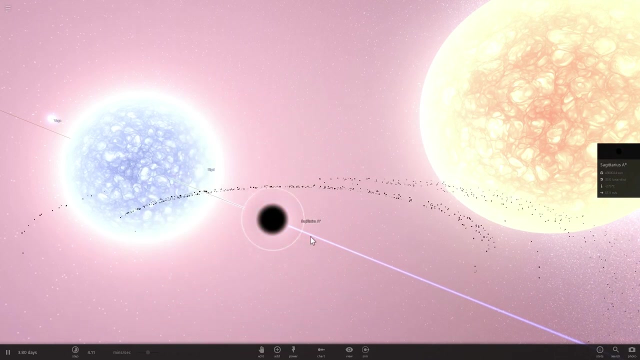 center of our galaxy called Sagittarius A is actually, uh, making a return, but it's still missed. wow, okay, I think it's just too large. that's probably why. so, as as these stars get absorbed, they release huge, massive amounts of energy, and all of this energy is released and this makes 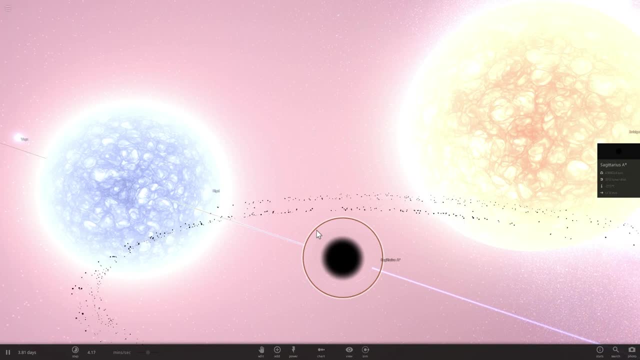 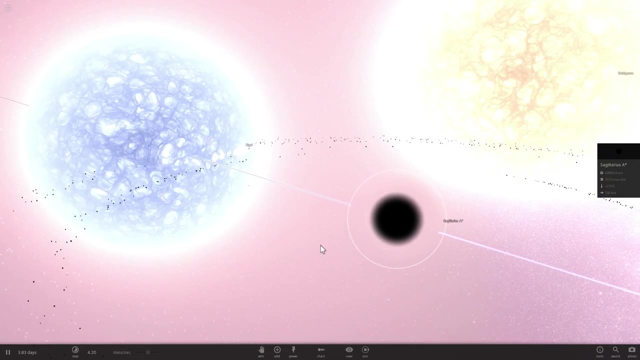 all of these objects called active galactic nuclei, all of these objects are the brightest objects in our universe, specifically objects called quasars and blazers, because, as I will explain to you in a moment, I'm going to show you how to do that. so, first of all, I'm going to 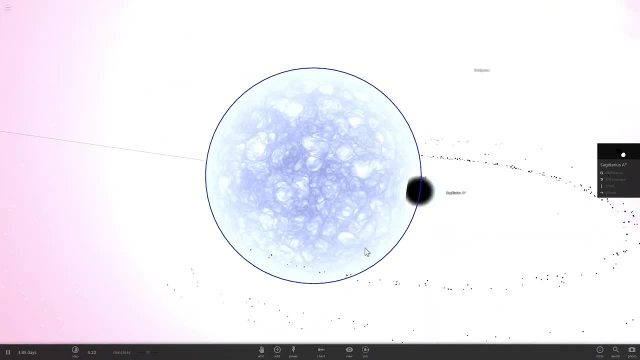 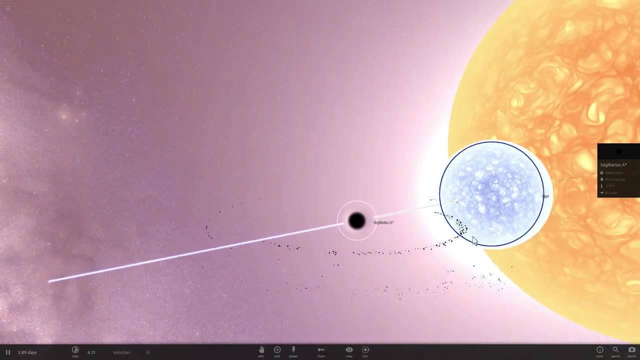 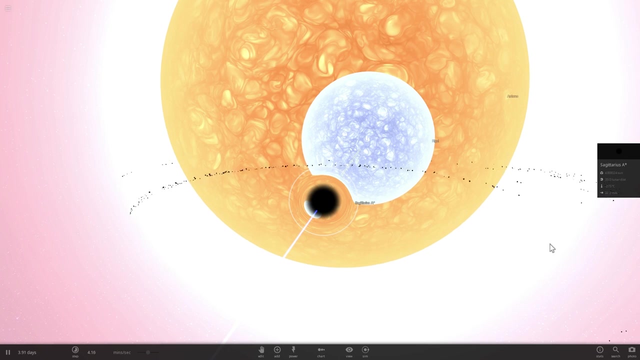 explain to you in a second. they create something called a super luminous stream, also known as relativistic jet, which basically is a jet of energy and particles. uh, that is so fast and so powerful that it basically emits a lot of various um, high energy particles and high energy radiation. 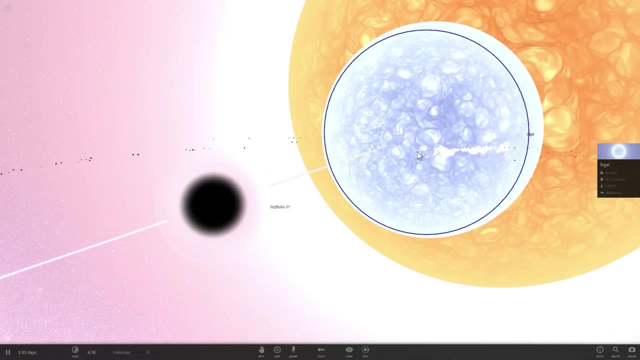 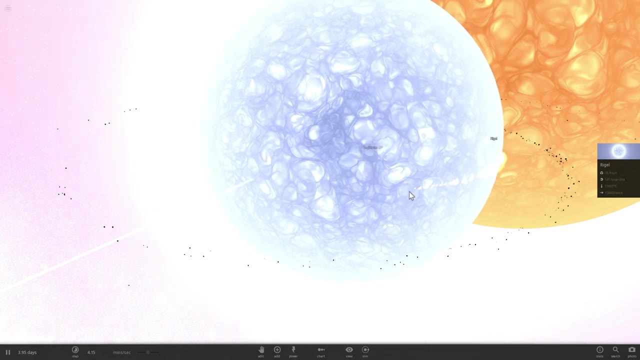 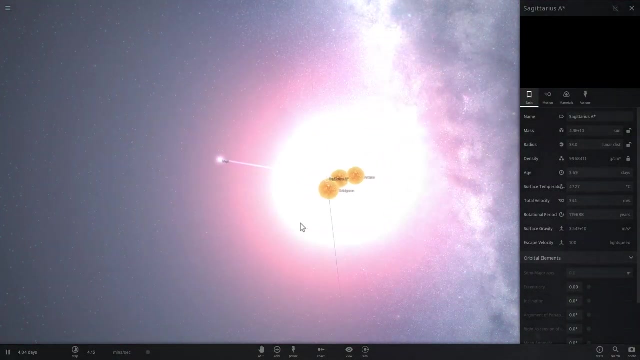 that we can then detect on earth. now, is this ever going to happen, Rigel? are you ever going to go and get swollen by that black hole or what? it's just being difficult. I think it's too large. I think big stars have trouble getting swallowed by a small black hole in this game, and that's okay, I'll forgive them anyway. so 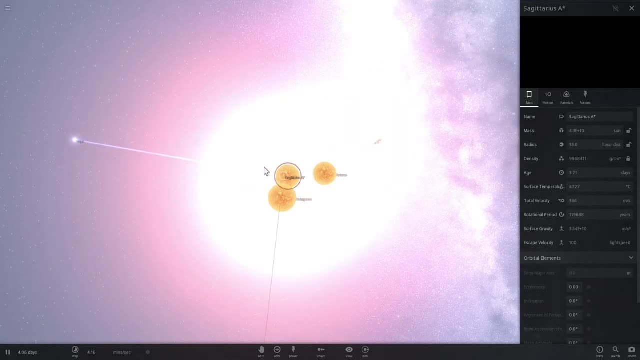 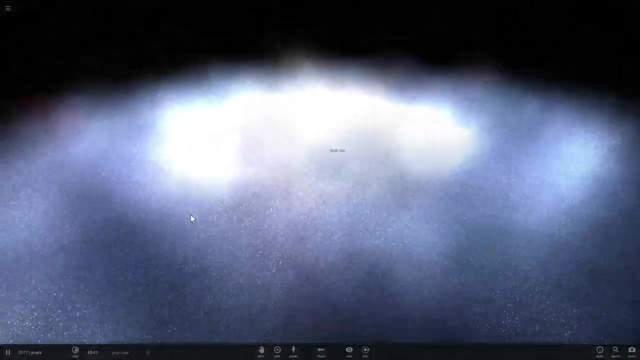 basically, this is kind of what happens: they get swallowed up and they uh emit a huge amount of radiation and energy. now, to try to simulate all of this, and try to simulate what an actual quasar looks like, we're going to use this um galaxy simulation. this is actually the one that's called. 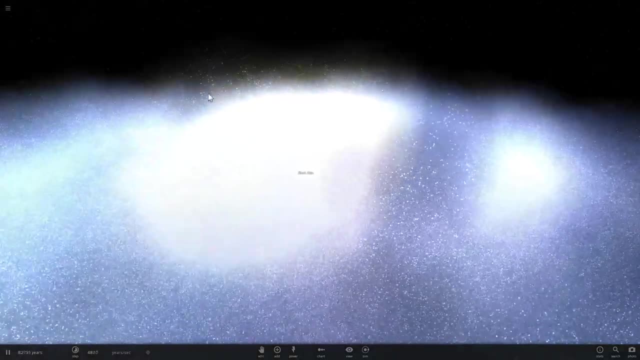 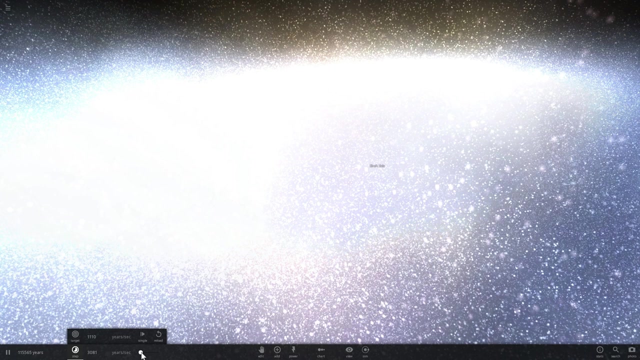 supernova in the galaxy. I just kind of removed the supernova and I removed the star, and we also are going to remove the central black hole. but before we do that let's slow down time, because if I remove the central black hole now, things will start flying away way too fast and 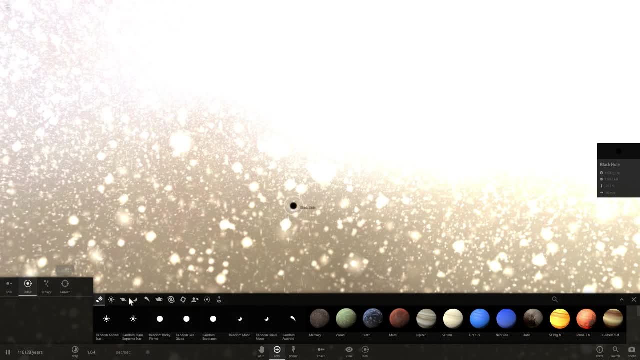 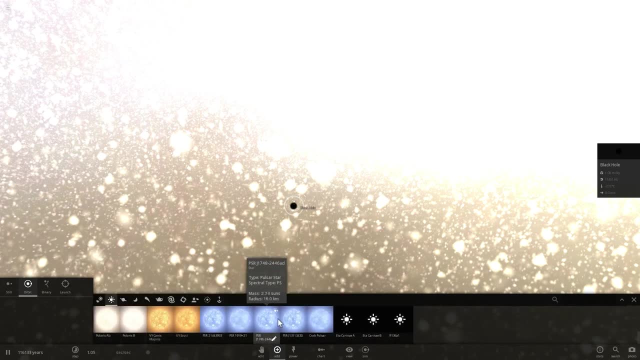 now, right here, next to the black hole, what we're going to do is we're going to place an orbiting white dwarf around it. I'm going to explain to you in a second why we're doing that. uh, so let's place a white dwarf and we're just going to pick this one right here, gj1221, and it doesn't really matter. 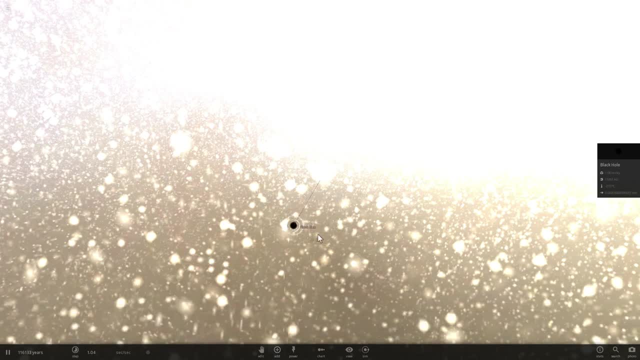 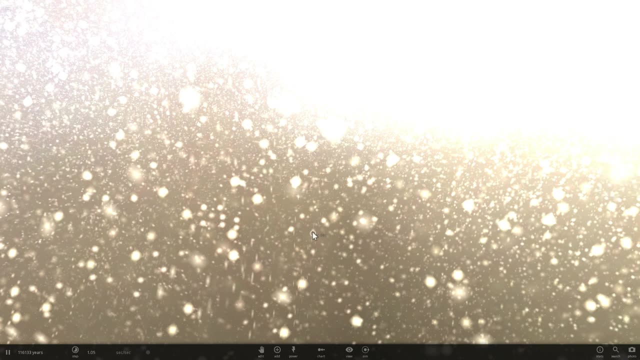 where you place it. just place it somewhere, and so this is just so we can actually create something that looks a little bit more like um a pulsar. so we're gonna now remove the black black hole, go into the uh white dwarf and play, make it total. 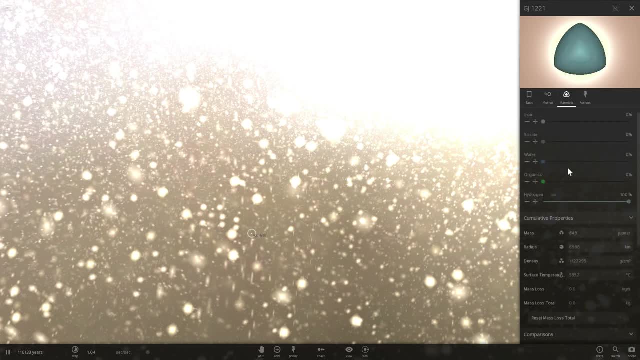 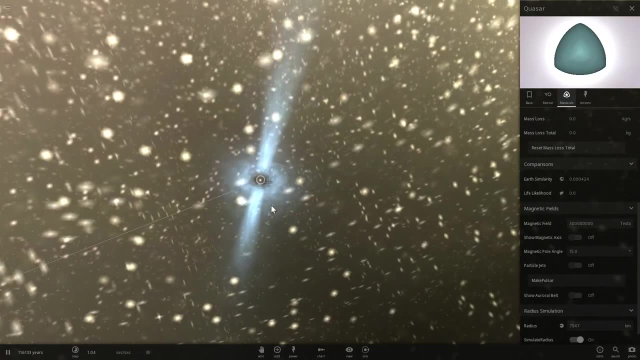 velocity zero, because we don't want it to fly away from us. now go to materials. I'm gonna use this new button called make pulsar. ta-da, this should have made a pulsar. did it make a pulsar or not? and here we go. I just made uh one and named it quasar. you can obviously name it whatever you. 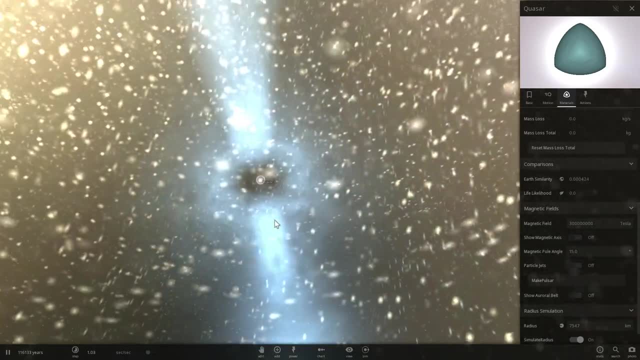 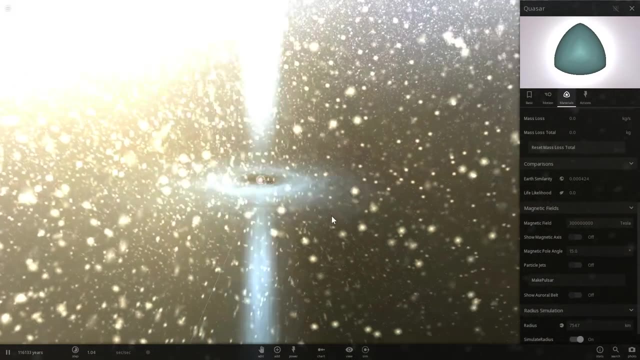 start of our manually made quasar slash Blazer. now next step is what we're going to do. is we're gonna? so? the reason why we're doing this is so that we can have these two jets coming out of the black hole, or pretend black hole, in this case going up and down. so this time, what we're going to? 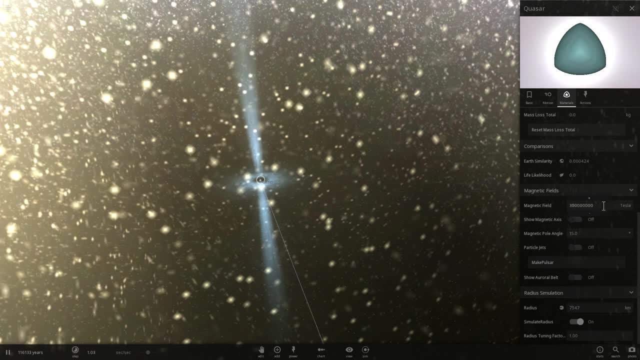 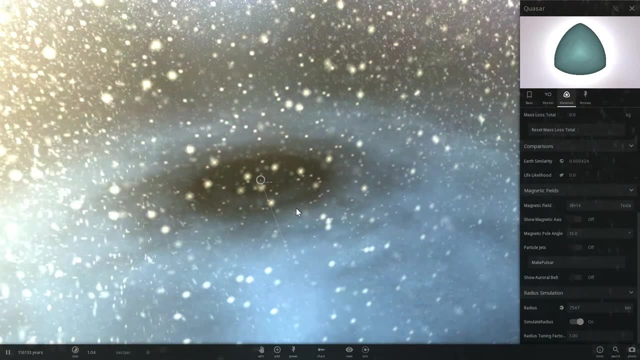 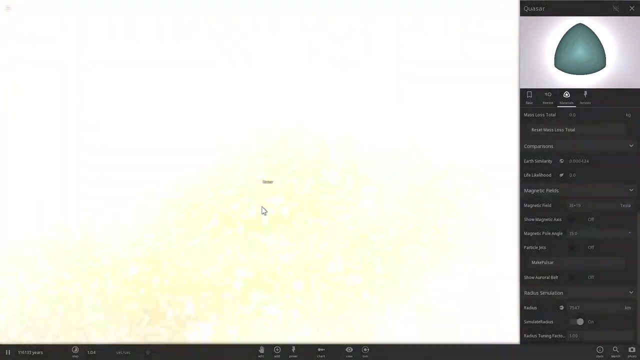 do is we're going to go down here and increase the magnetic field by like a factor of a million. so let's just add six zeros in here and this will hopefully give us enough magnetic. no, even more than four. let's actually add maybe a few more zeros until this becomes a very prominent. there we go. 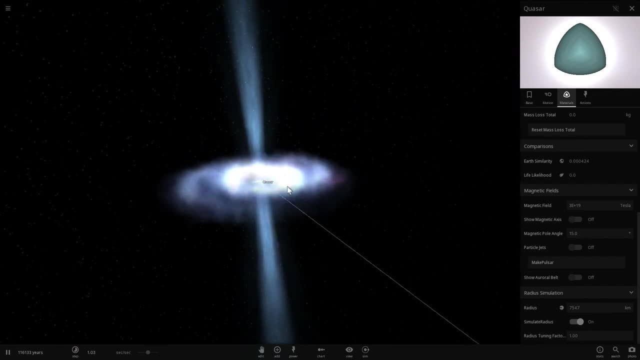 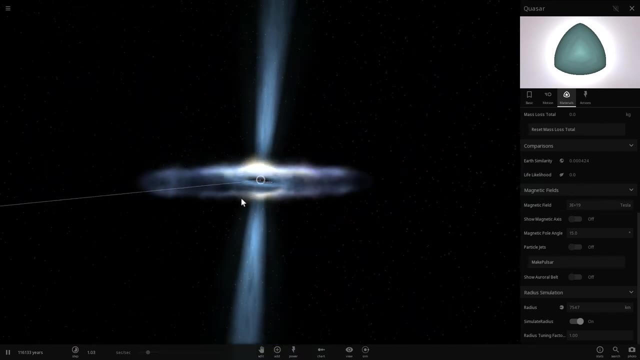 very, very prominent looking stream. this is what I was looking for. now, as you can see, there is actually two streams coming out of this uh, particular Galaxy, and this is essentially what a quasar would look like, except maybe, I think it would be maybe a little bit more straight than. 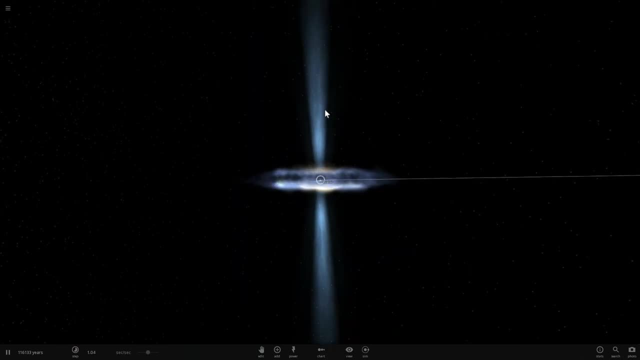 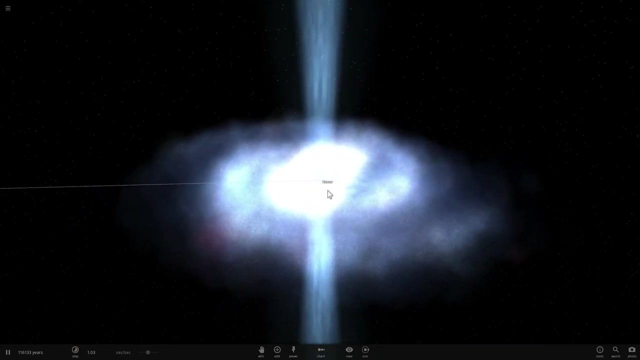 that. so let's see if we can straighten this out a little bit. okay, I think this is straight enough. so let's just talk about what quasars and Blazers are and how they work, and how they work and how they are in terms of us seeing them. so imagine a Galaxy, and right at the center you have this. very, very. 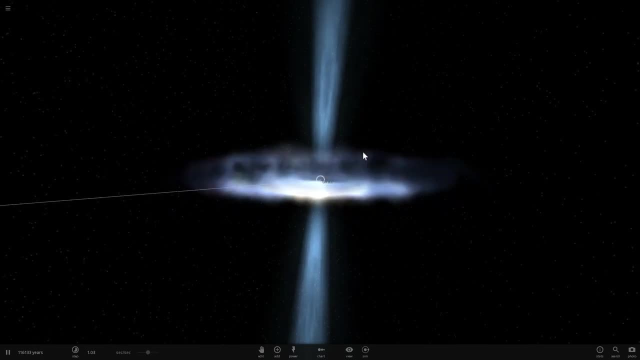 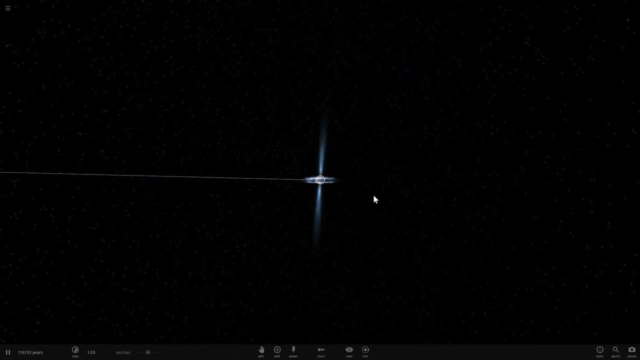 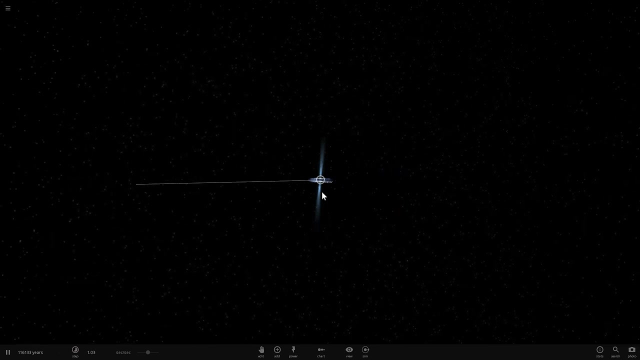 active black hole that is absorbing a lot of matter, and a lot of this matter is propelled up and down in this way. now, if you're looking at it from a distance, from sort of like this, this angle, you're observing something called a radio Galaxy. radio Galaxy is essentially a. 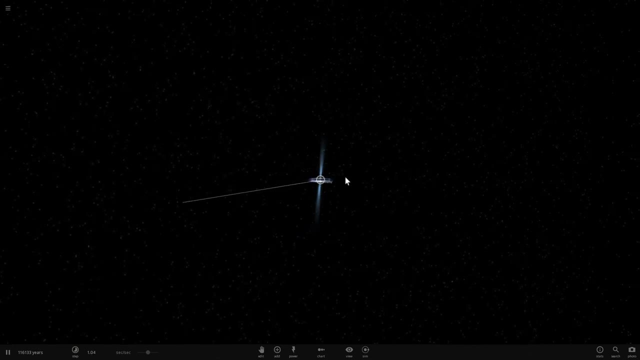 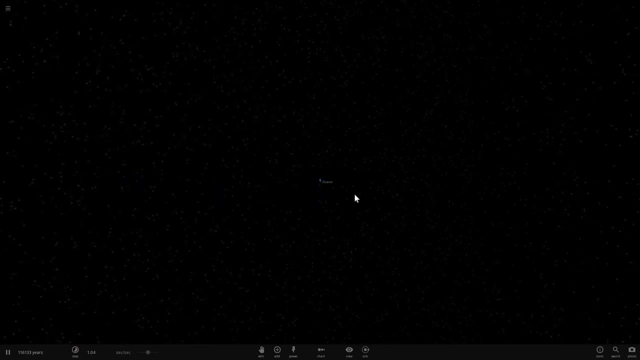 Galaxy that is emitting a lot of radio waves, a lot of, um, really interesting uh spectrum, of whole sort of radiation, and if, from a distance, it would obviously look more like this: it's not particularly bright, it's not particularly interesting, or I mean it is interesting but 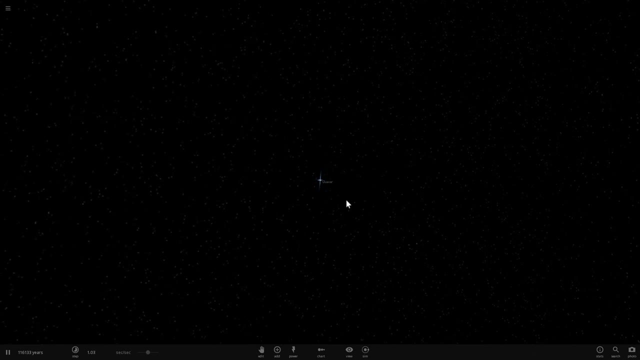 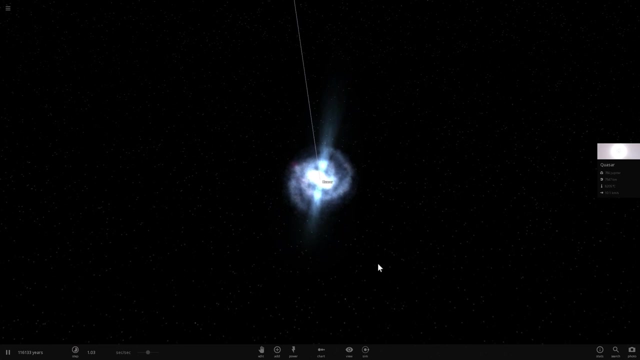 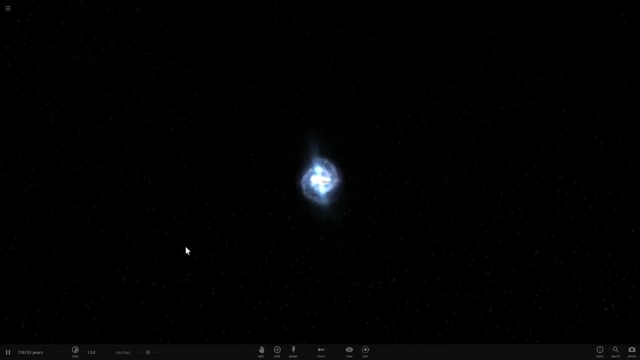 it's not, uh, specifically that interesting compared to quasars and Blazers. now, some of these galaxies are under this angle to us and they show us their face a little bit more. now. this right here, anywhere sort of any sort of angle that is in this way, is called a quasar, so quasars are a lot more bright. 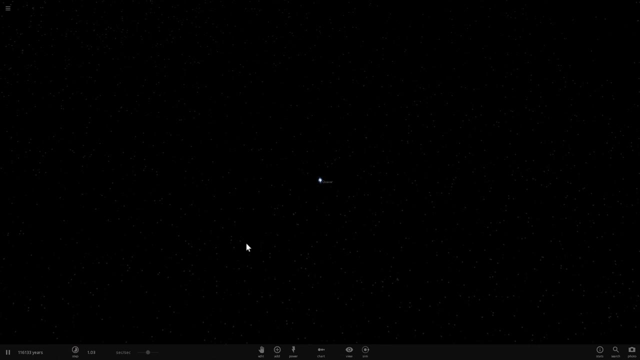 and a lot more interesting in terms of spectrum that we receive. we get a lot of different uh high and low frequency radiation from them. we'll get a lot of x-rays. we get a lot of gamma rays. we also get a lot of real interesting effects that sometimes make it look like the light coming from them is. 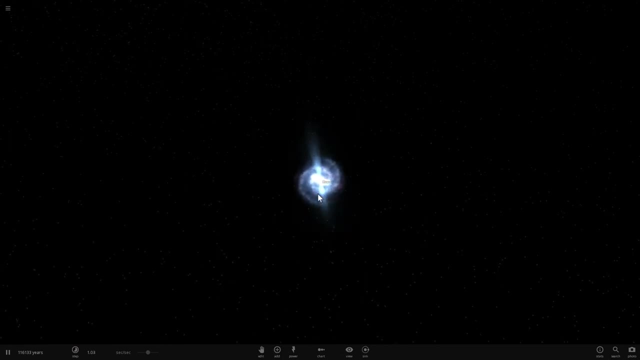 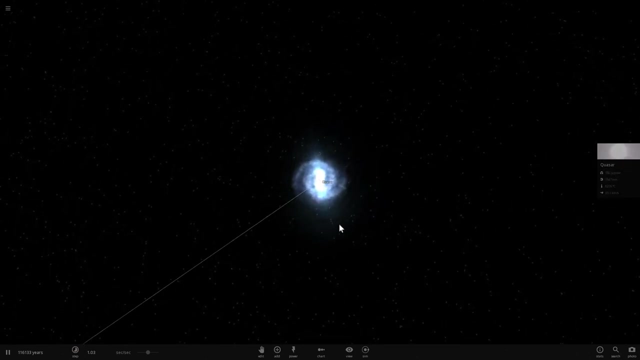 actually traveling at faster than speed of light, and that's because they're so far away that they're creating this sort of effect called super luminous emission. now, this is what happens when you have, um, something that comes out of, uh, the black hole at almost the speed of light, but because you're observing it at a slight angle, it in overtime, over 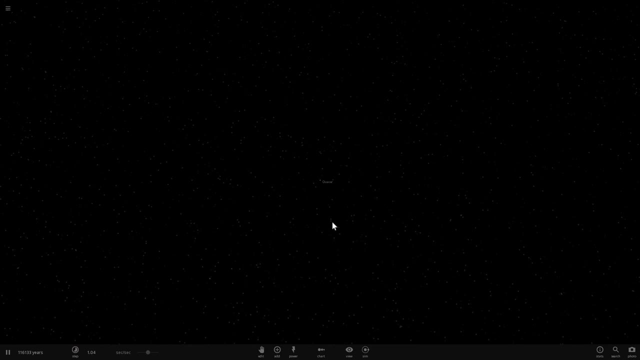 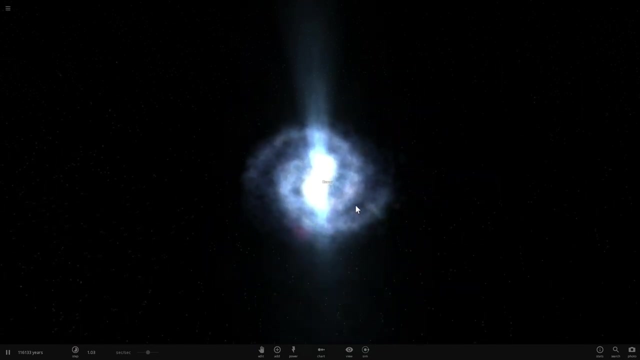 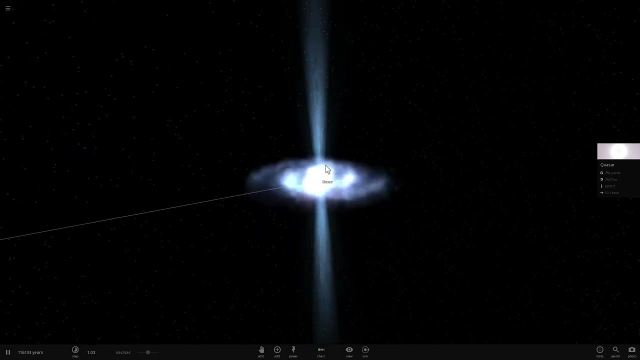 sort of years and millions and millions and billions of years of travel. it essentially kind of looks as if this object or this light was traveling faster than the speed of light. unfortunately, this is a optical illusion, not an actual physical phenomenon. so, and what I didn't mention is that a 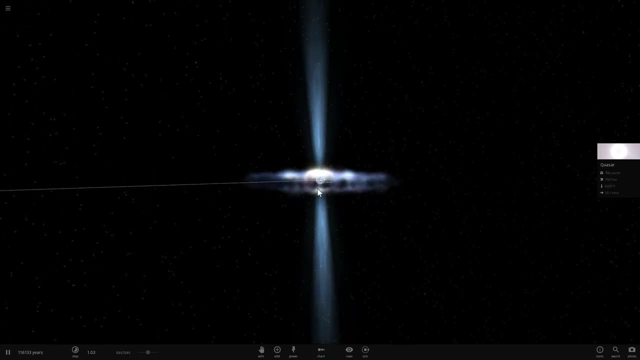 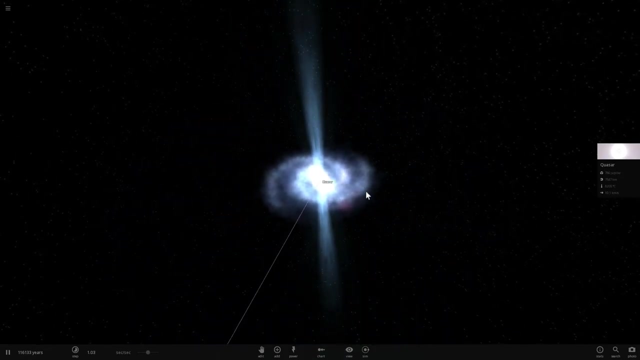 lot of the stuff that comes out of these jets, uh, so coming from the black hole up and down, a lot of that's very close to speed of light. It's about anywhere from 95% speed of light to about 99% speed of light. so it's probably the fastest sort of particle accelerator that we can find in the 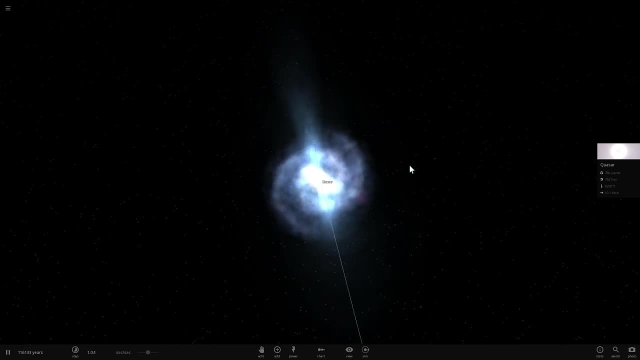 universe. Now that's quasar and this is what quasars look like. So basically, it's when it's under a bit of an angle, but not exactly straight on. Now what happens if you look straight in the? 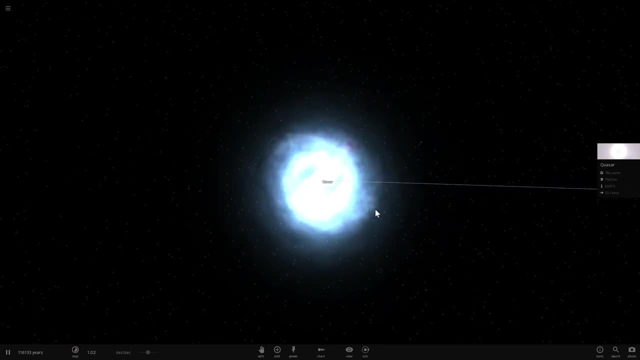 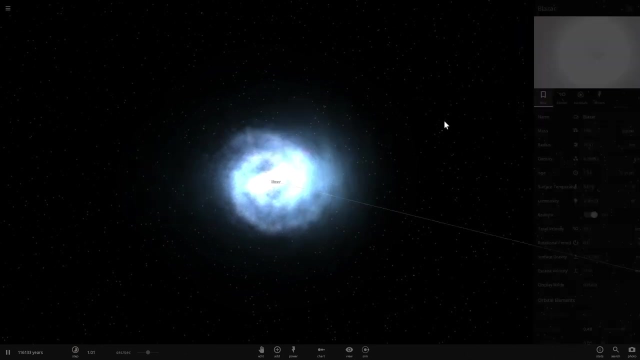 middle, And this actually is what we're really interested in right now. This is actually what the most interesting object, in my opinion, is, and this is, of course, called- and I'm going to rename this now- this is what you would call a blazar, So if you're staring right in the middle, 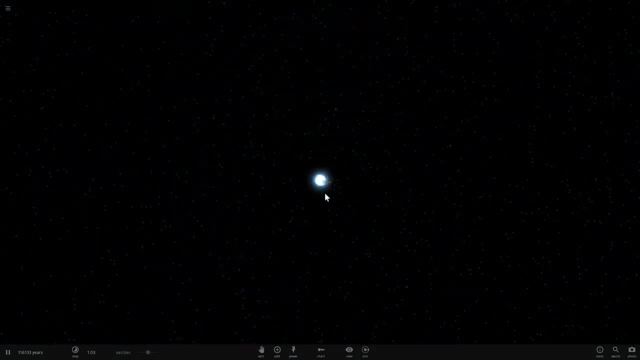 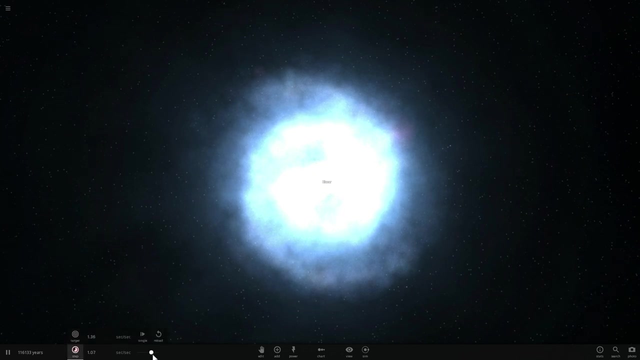 and you get this absolutely ridiculously bright object. this right here is what blazars are, So essentially it's just a different angle of looking at things. So it's still the same object. It's still a super active galactic, nuclear because of the black hole that's absorbing a lot of this. 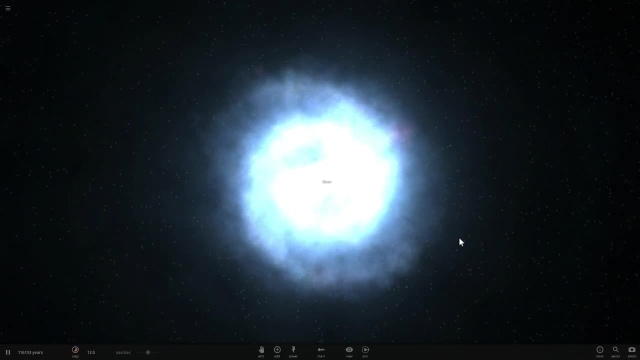 light and I'm actually going to Accelerate time a little bit so you get to see what it looks like And if you're staring right into the ray, you get blazar. There's not that many that we have found, because having a chance, 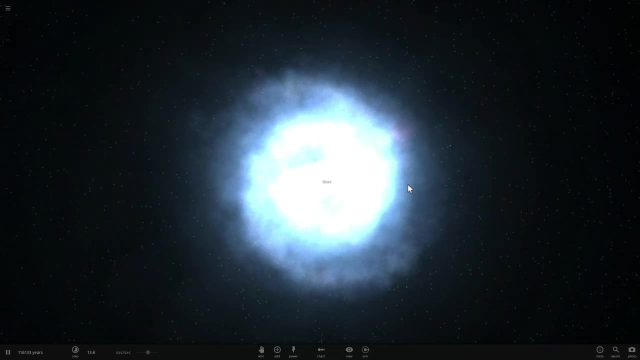 of a quasar aligning itself so it stares directly at our planet is actually relatively low, And so there is not that many blazars that we found, but we did find something like a million of different quasars. Quasars are a lot more common because it's more likely that you'll be observing these. 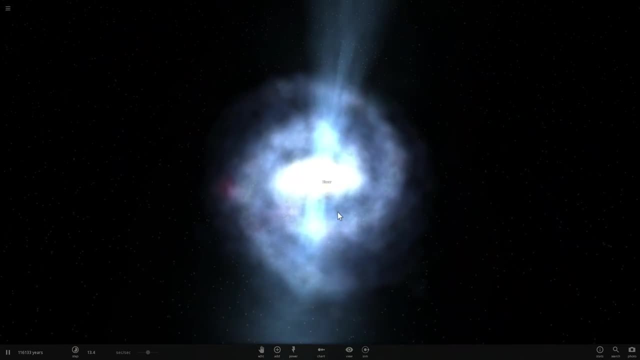 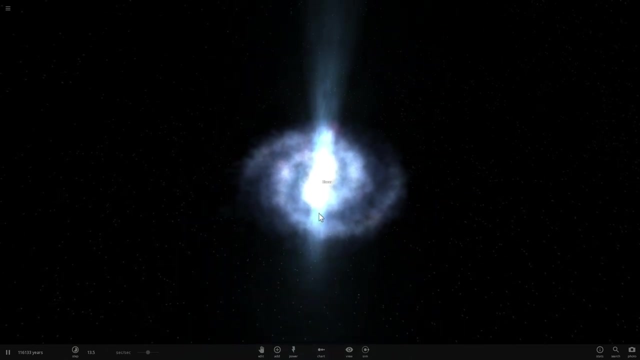 active galactic nuclei at an angle not exactly Staring right in the sort of eye of the black hole, but you're going to be more likely to observe them this way, And obviously the radio galaxies are also very common, where you're basically just 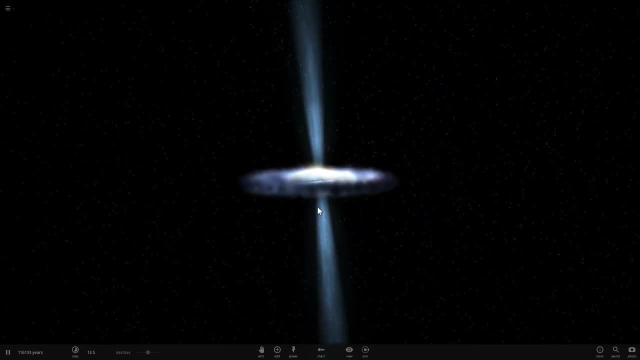 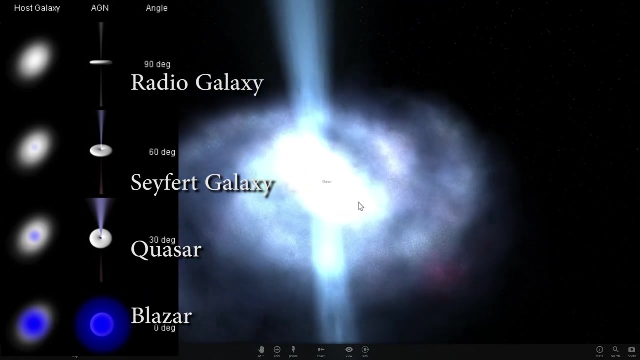 looking at them from the side. So here's the summary of everything here. This is essentially how they are classified today and what we know about them today, So they're not particularly mysterious anymore. They used to be very mysterious objects. We actually could not really. 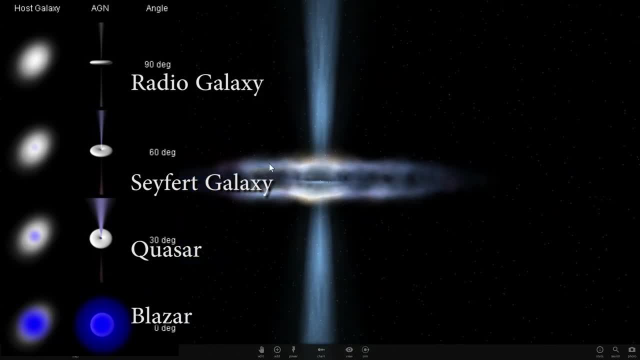 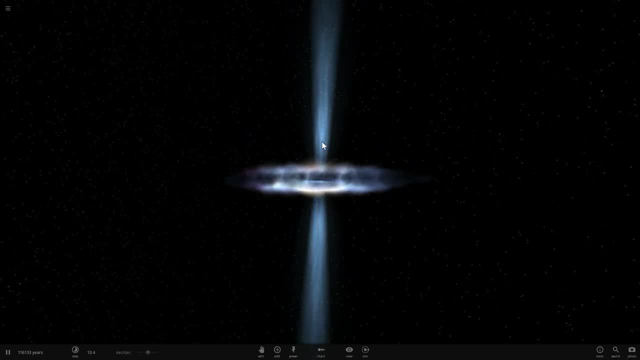 understand how they work and what they do, but today we are absolutely convinced that they're not. It's because of the supermassive black hole, and the supermassive black hole creates these jets- particle jets- that release energy really fast, And we actually even have pictures of them. 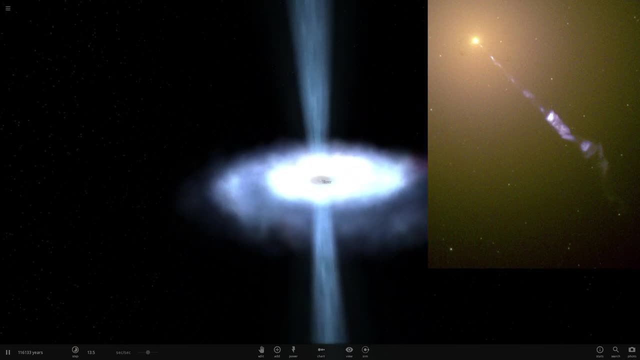 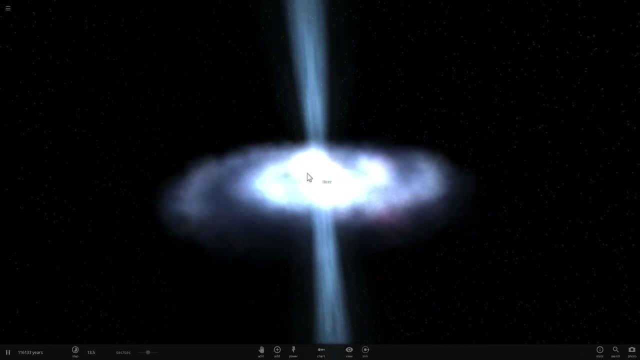 from Hubble telescope. Here's one, for example, where you can actually see the jets coming out of the black hole, And there is actually some recent discoveries when it comes to quasars. We've actually discovered some really cool things about them. One of the things from last year: 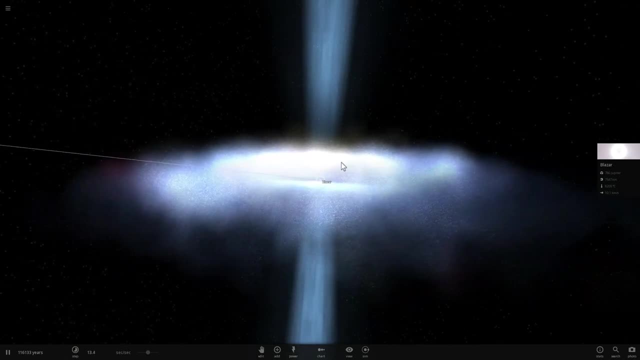 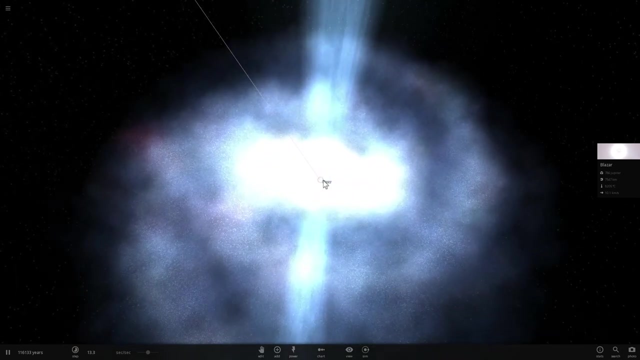 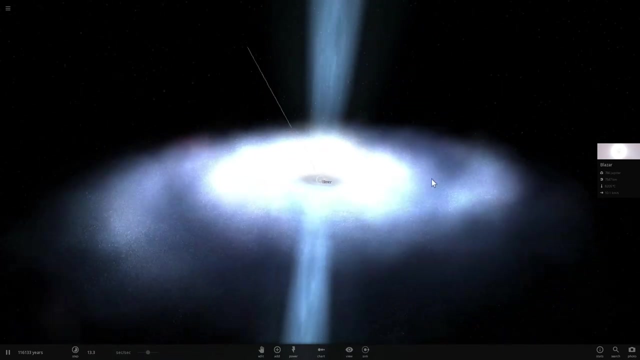 actually from 2014 and 2015,- is that we've discovered that a lot of them have such a varied luminosity- In other words, they change luminosities so fast that we realize that they can change from active nuclear galaxy to basically a quiet or inactive galaxy within years, Not even. 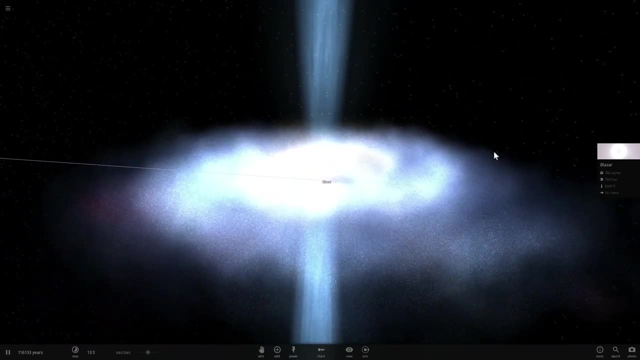 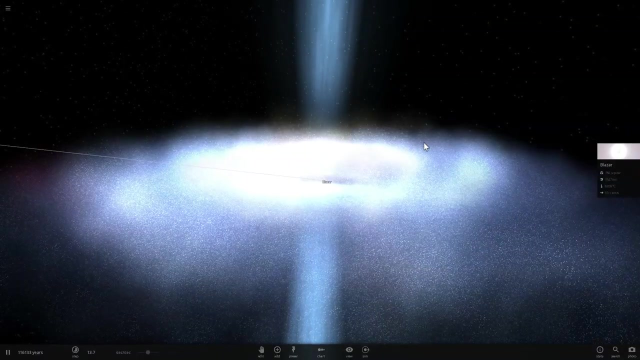 millions of years or thousands of years, but within our lifetime. So one of the scientists that I'm going to be talking about in the weekend's video- because this is actually recent news, and her name is Stephanie Lamassa, from NASA, And I'm going to be talking more about her during the 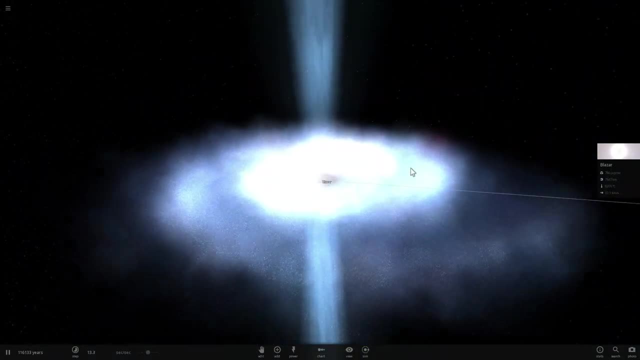 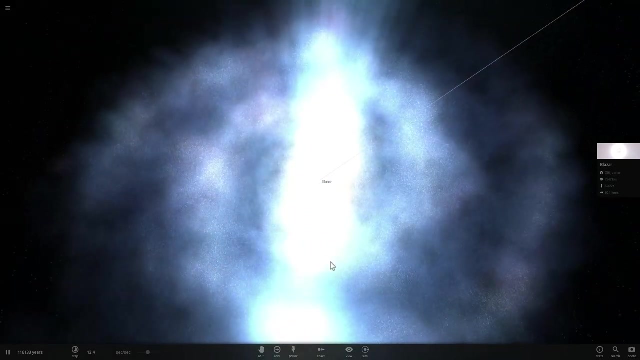 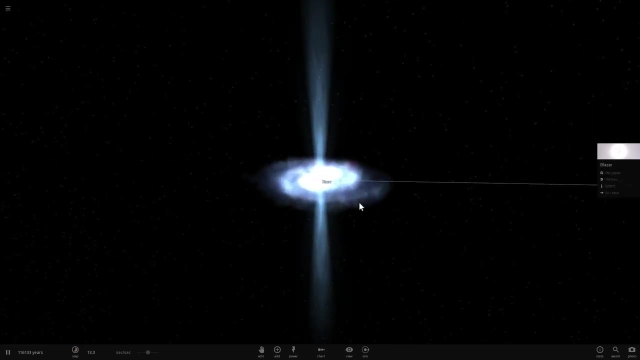 weekend news, with what the math when we talk about space news? But basically, yes, she discovered that there is a quasar that she found that changed from being super, super bright to almost invisible within 10 years, And now we found even more of these. So we know that their luminosity, their activity, their actual sort of 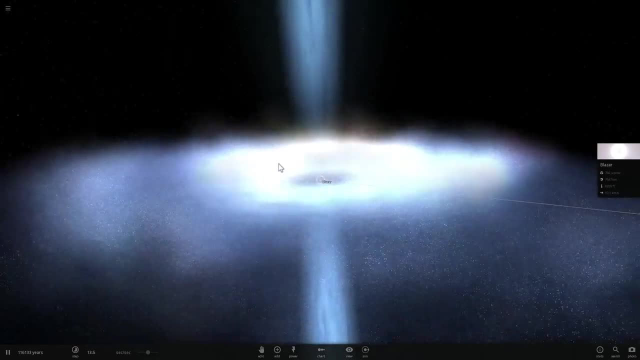 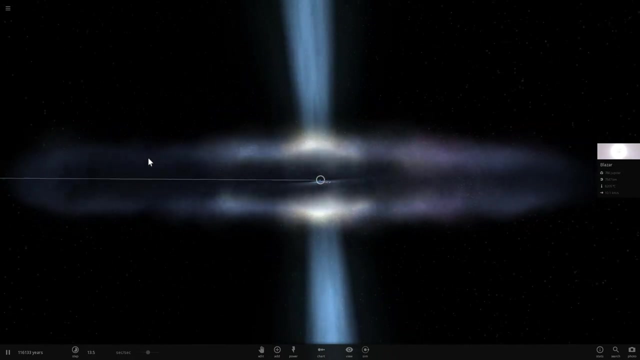 coolness, their black holes that absorb all this energy and release it can change within years And it's a very sort of volatile process that can change this from a quasar to a normal galaxy within several year periods And the other thing that's very 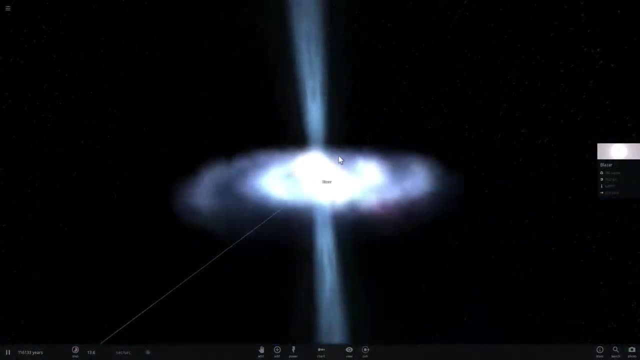 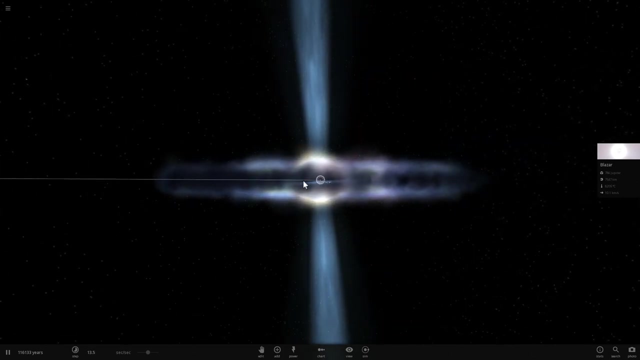 interesting- that was found very recently as well- is that our galaxy also emits these rays, but they're not as prominent. So actually all galaxies emit these rays. When a black hole in the center starts absorbing anything, it starts emitting these rays, And we actually discovered that our galaxy has a 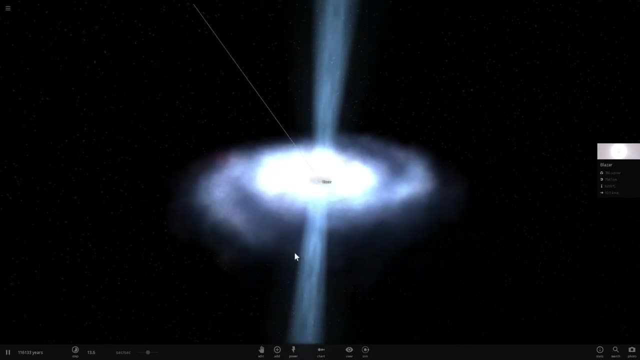 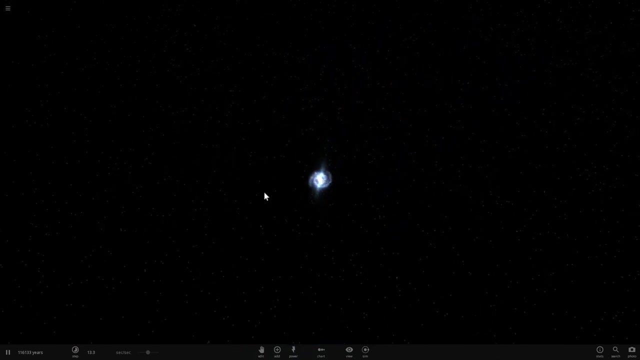 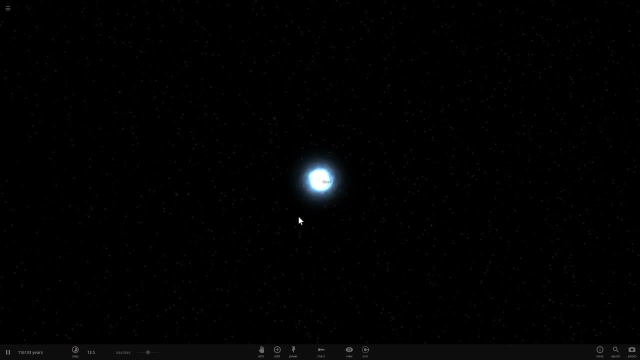 very, very slight sort of emission of these two rays. And so if there's a galaxy somewhere far away inhabited by some super smart species and they're actually looking at our galaxy and they're seeing this, they're probably also might even be wondering, so what's going on in there? and you know, is there? 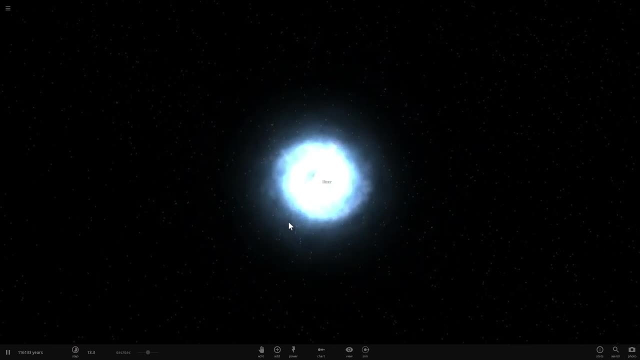 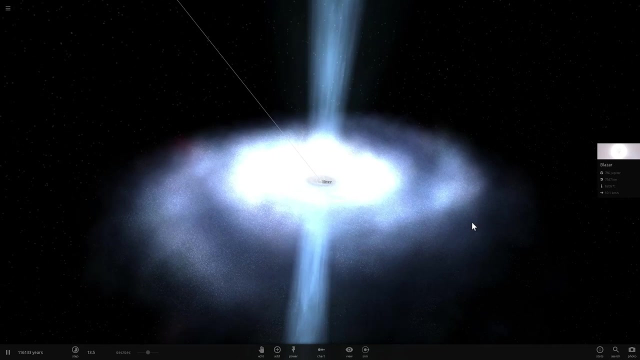 anyone in that particular galaxy that is alive and is intelligent and uh. but one thing i didn't mention is that a lot of the quasars and blazers we're observing right now are ridiculously old. remember, the light travels at speed of light and the light we detect from the quasars and blazers. 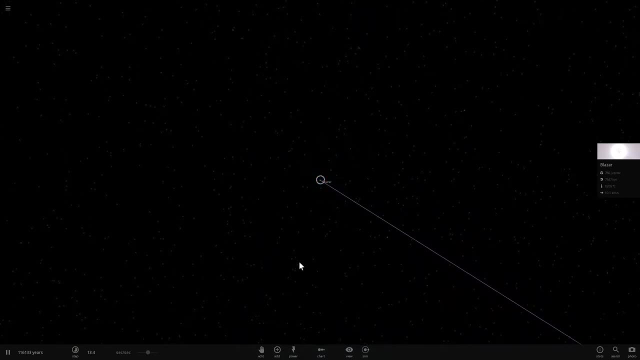 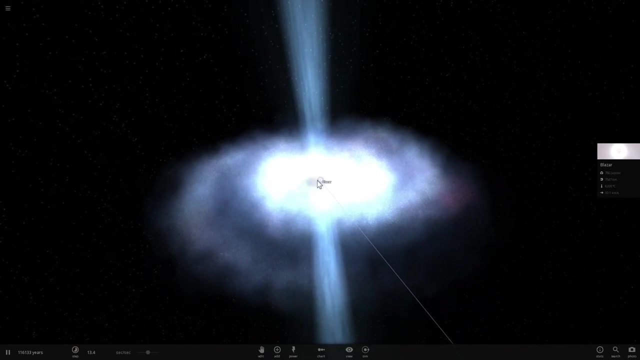 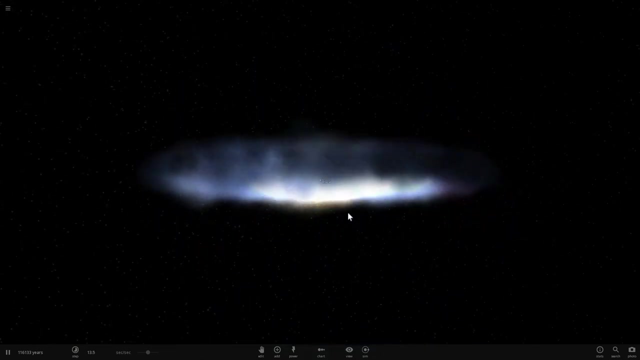 that we see today is billions of years old, so, in other words, what we are seeing is no longer there. they are probably just normal, regular galaxies that don't even have this anymore. they probably just look like this or maybe something completely different. they might even be a completely 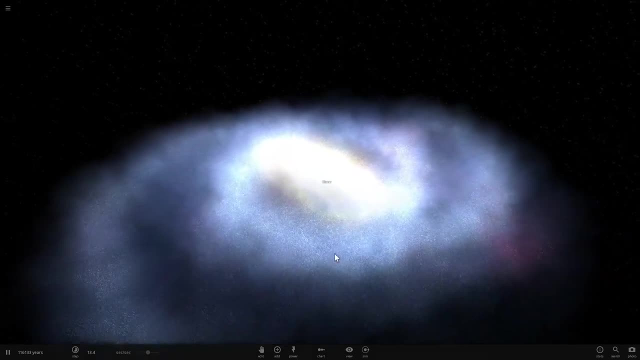 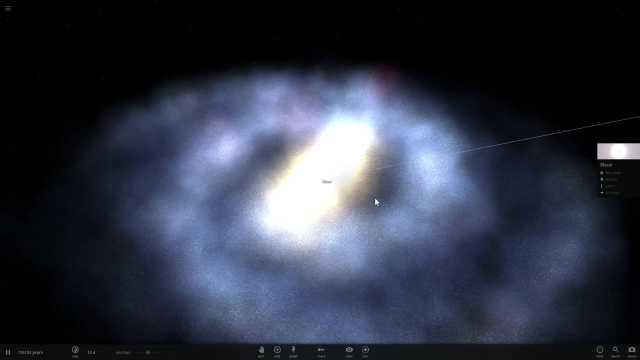 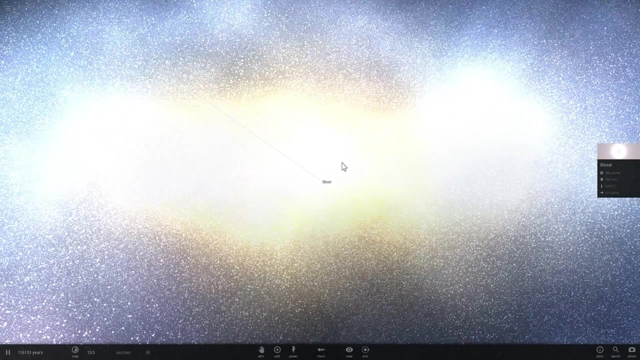 different shape by now. uh, so the blazers and quasars are not really permanent objects. they come and go all the time, and even our galaxy may one day become a blazer or a quasar or basically, will acquire active galactic nuclear if a lot of stars come within the central area of the black. 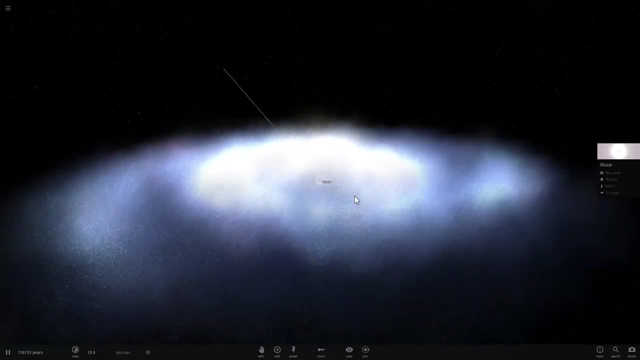 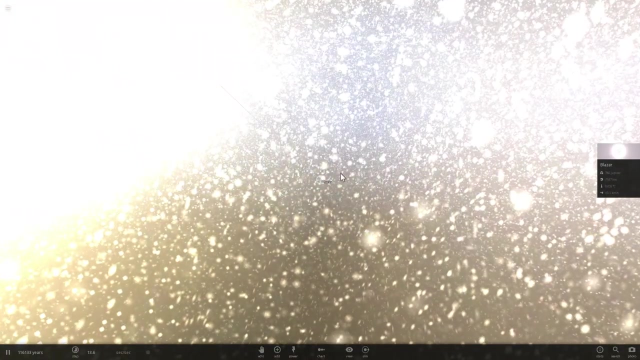 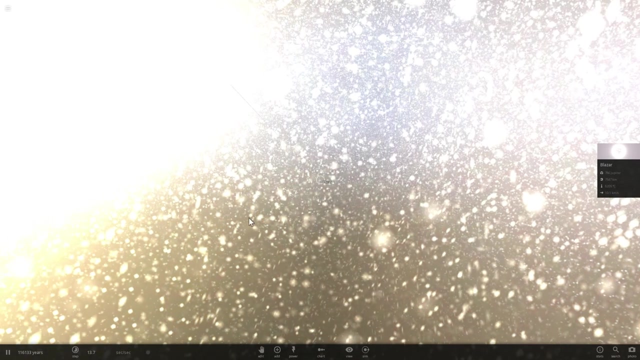 hole, or when andromeda galaxy comes to visit and collides with our galaxy. if a lot of stars approach the supermassive black hole that forms as a result of the merge of two galaxies, we might also get, or we might also become, a blazer or a quasar. so yeah, a lot of these objects come and go. 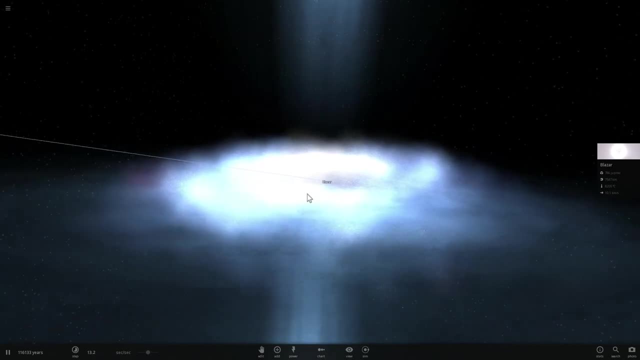 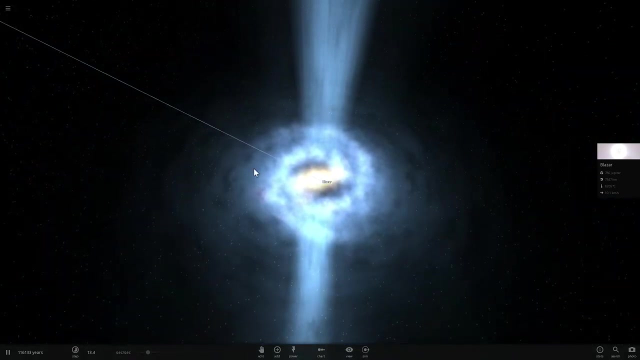 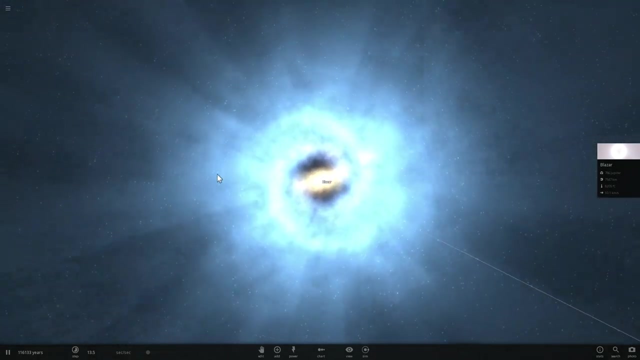 and, as i mentioned before, we currently have a list of approximately a million of quasars and approximately a thousand five hundred blazers. in other words, there is approximately specifically 1580 objects as of late 2015 that are staring exactly at us. in this fashion, we can actually 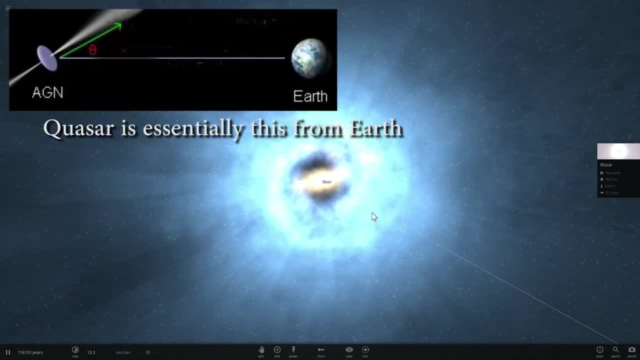 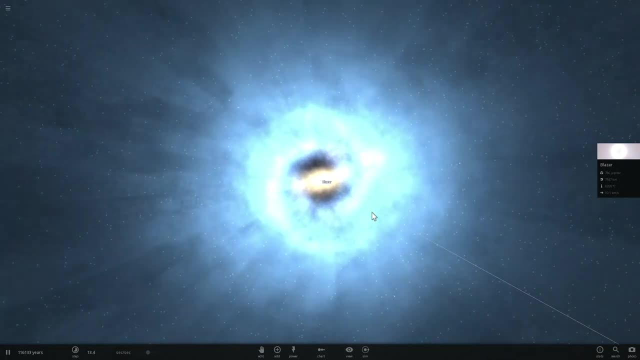 see them and they're super bright. they're so bright, in fact, that if you, uh, if you watch my luminosity video and that, where i compare different luminosities, their luminosity is minus 26 to minus 26, and that's the luminosity of the galaxy. and that's the luminosity of the galaxy, and that's.